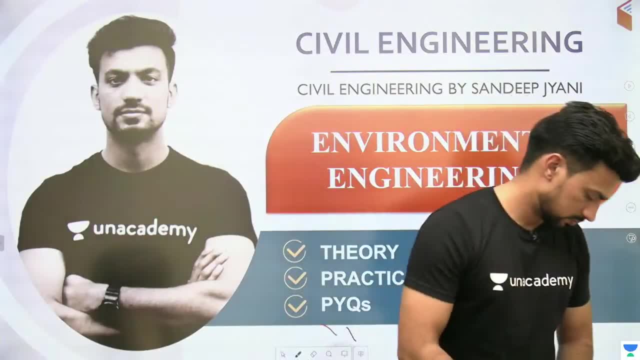 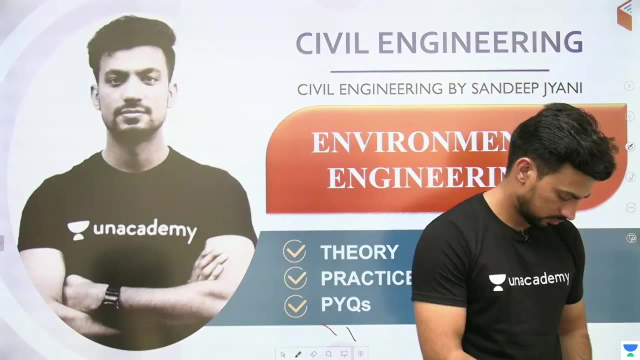 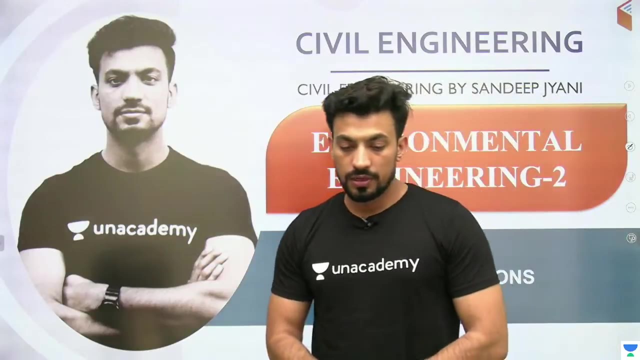 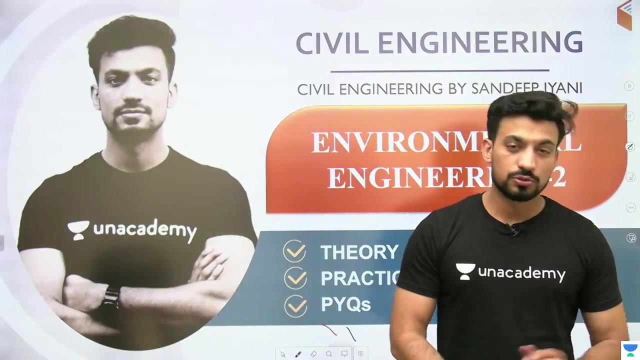 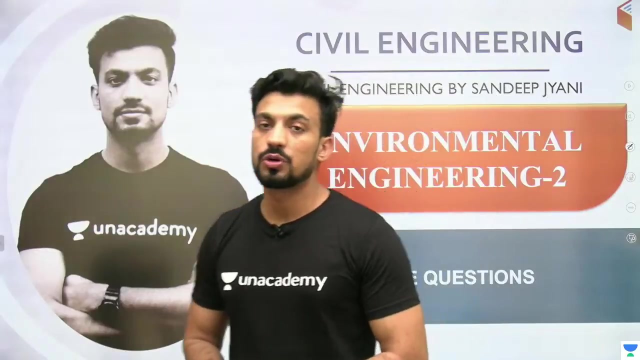 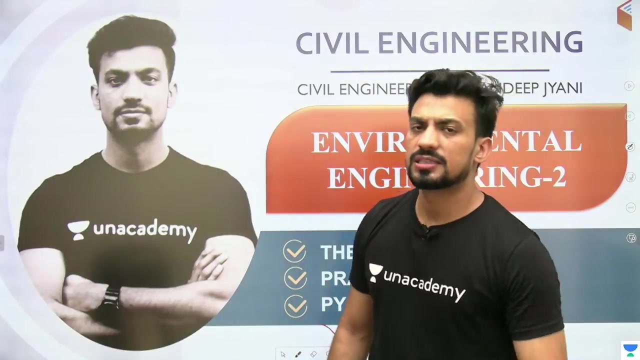 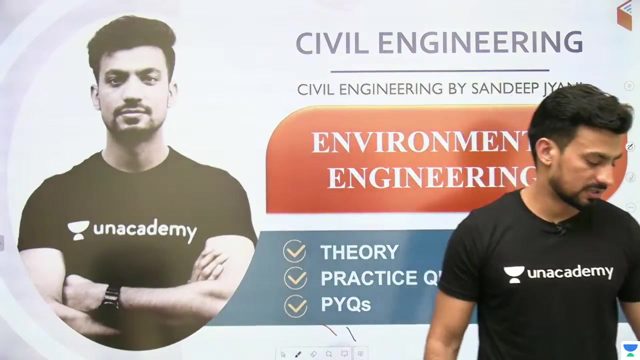 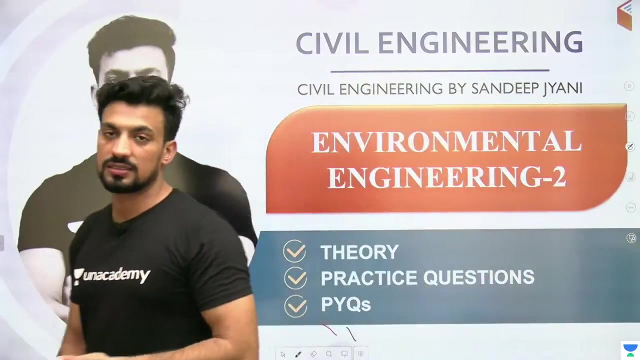 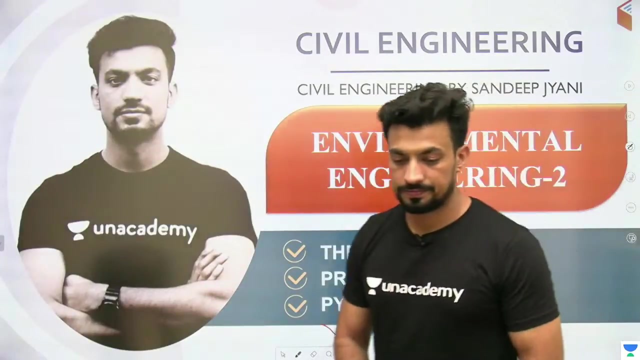 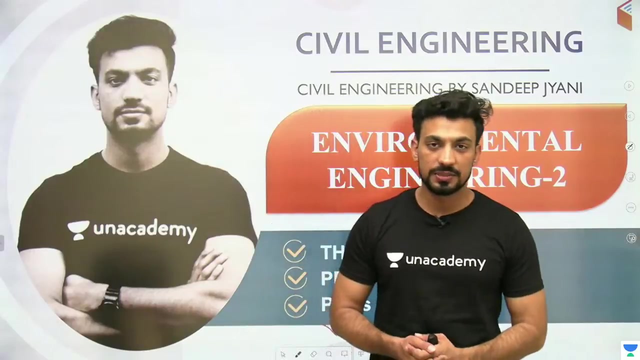 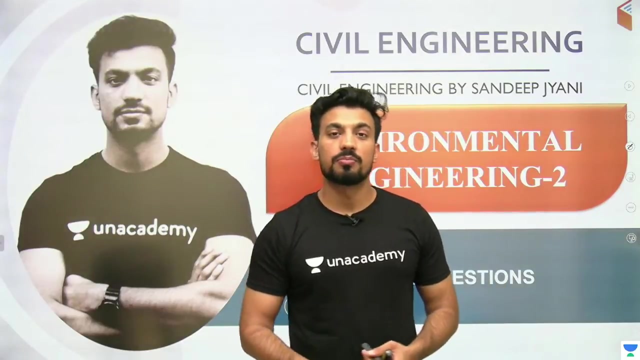 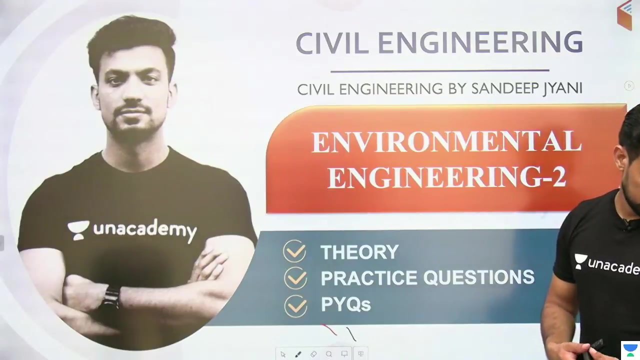 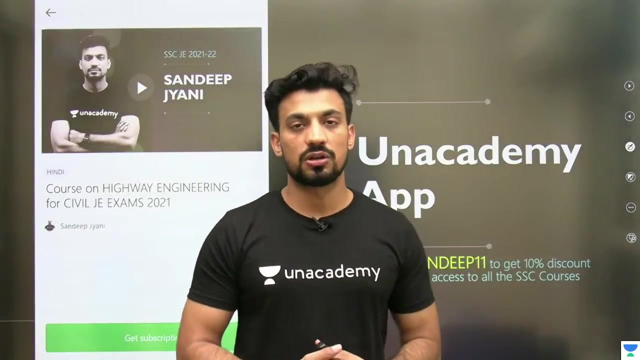 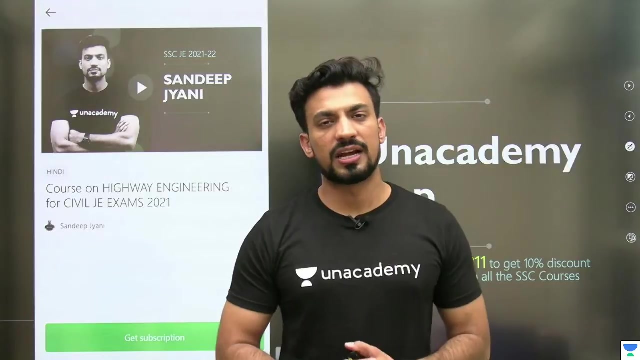 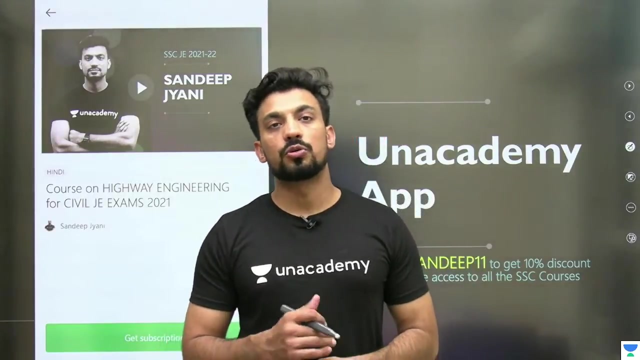 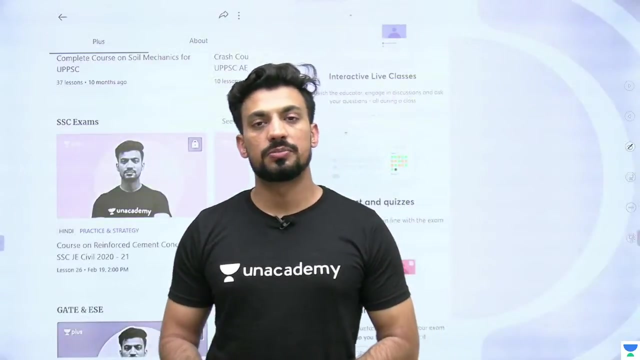 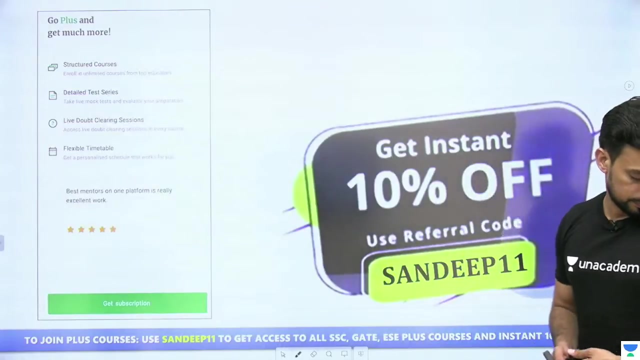 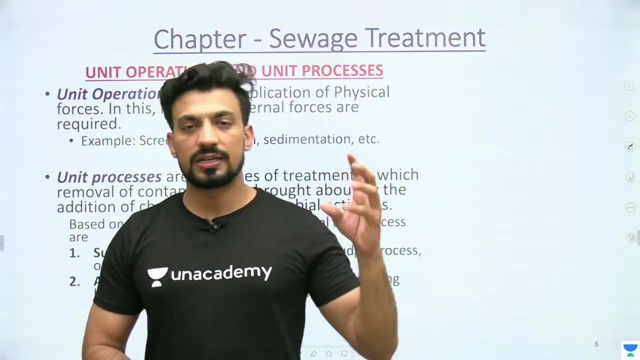 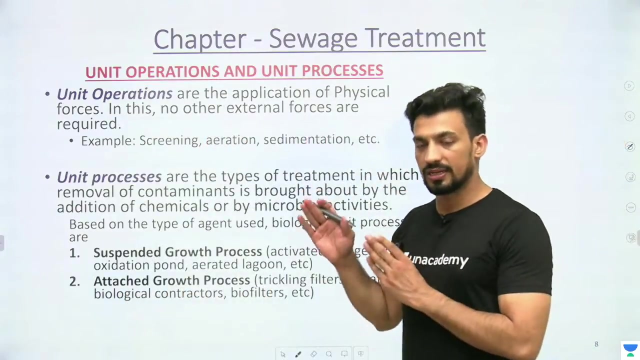 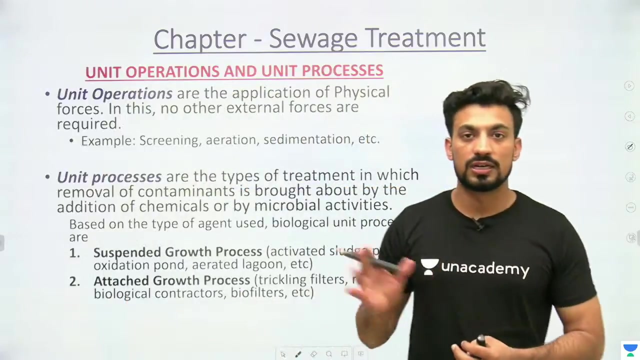 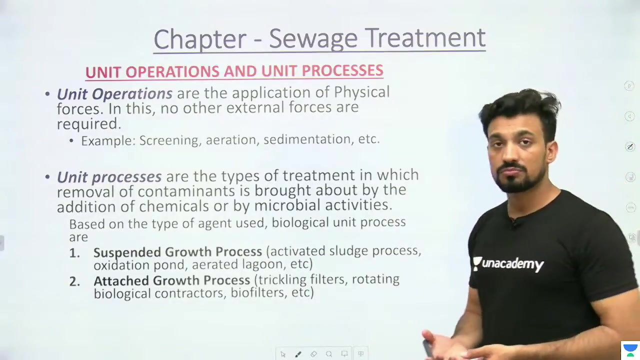 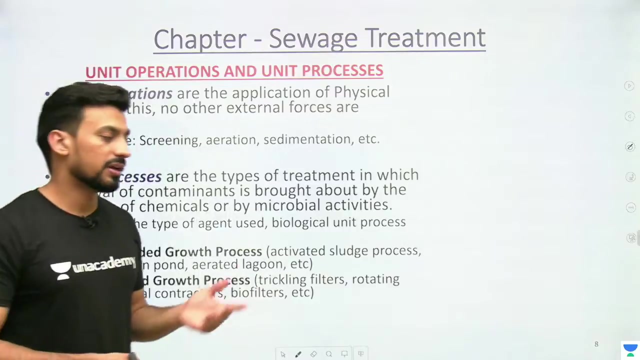 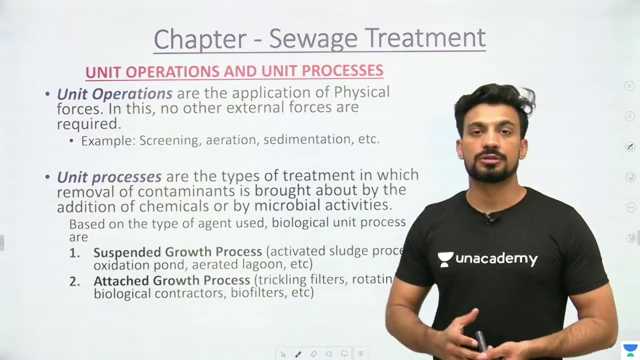 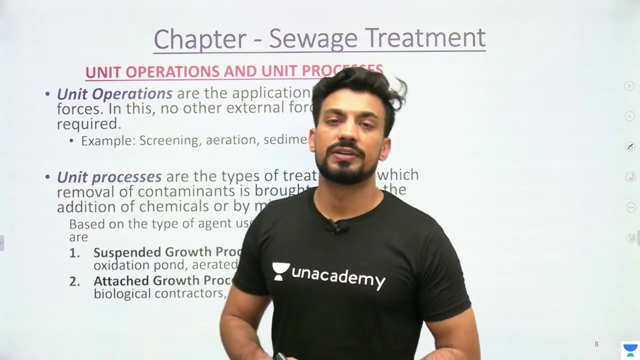 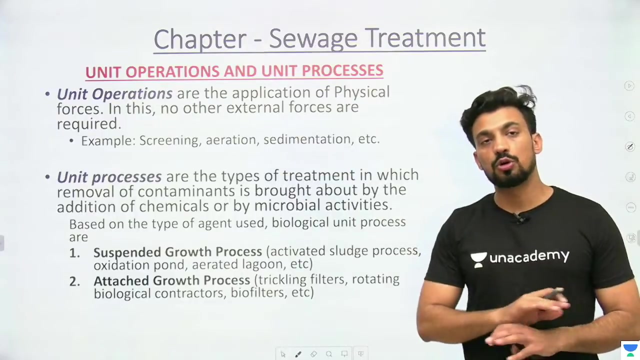 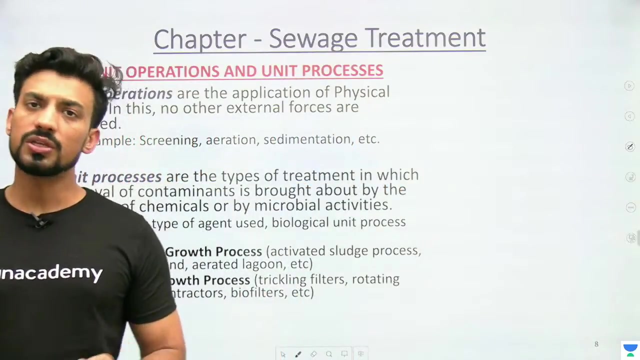 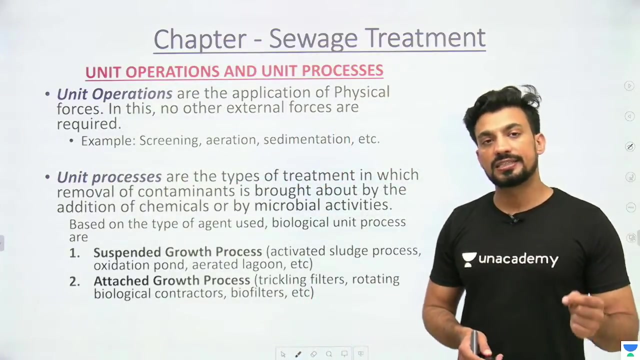 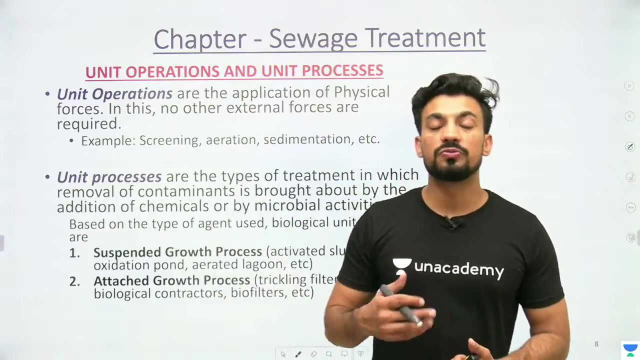 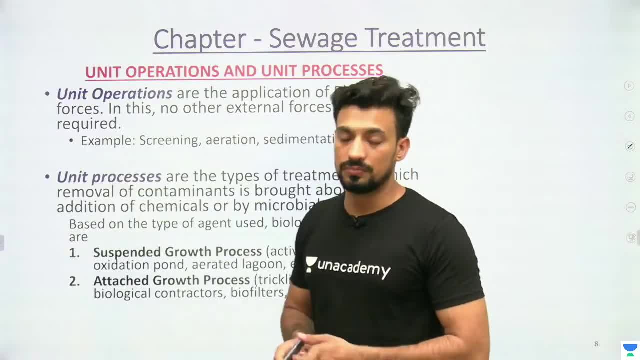 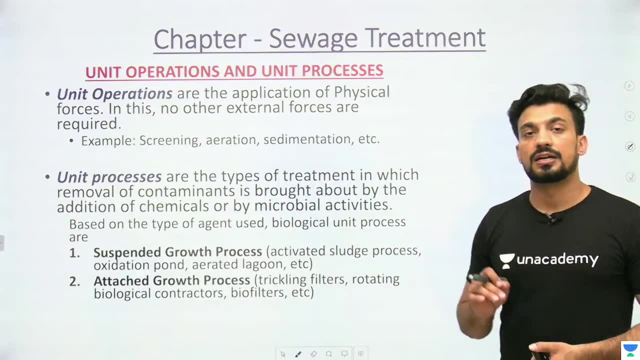 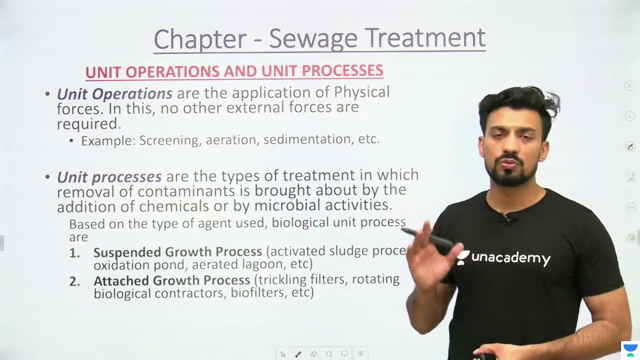 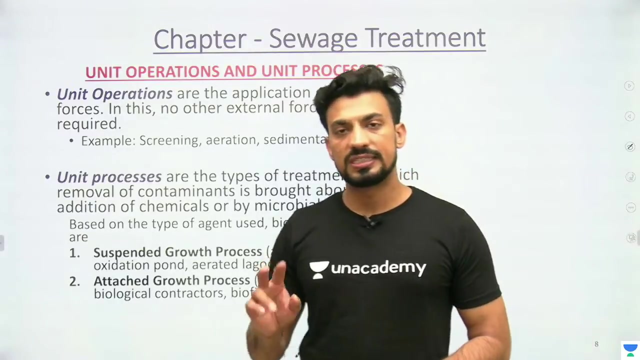 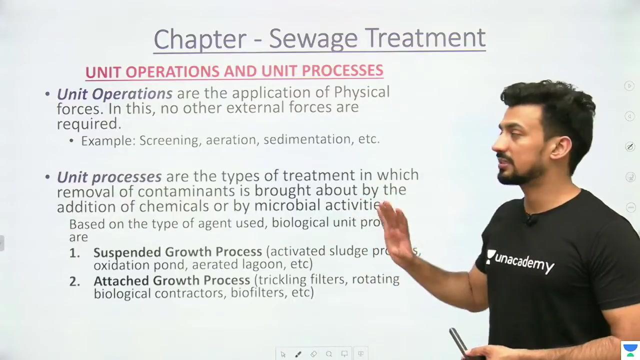 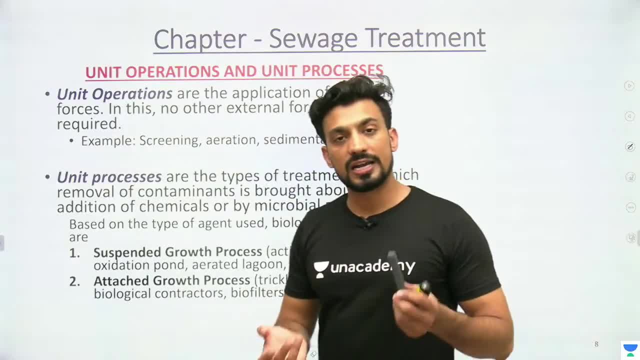 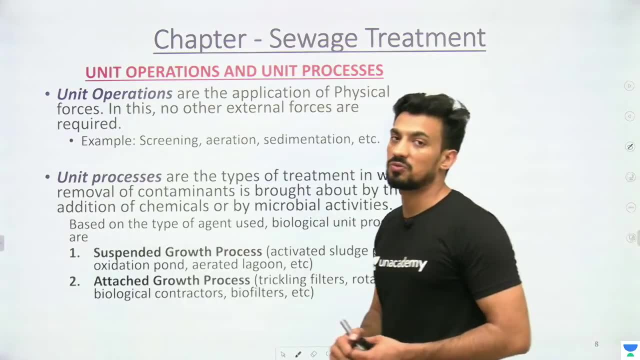 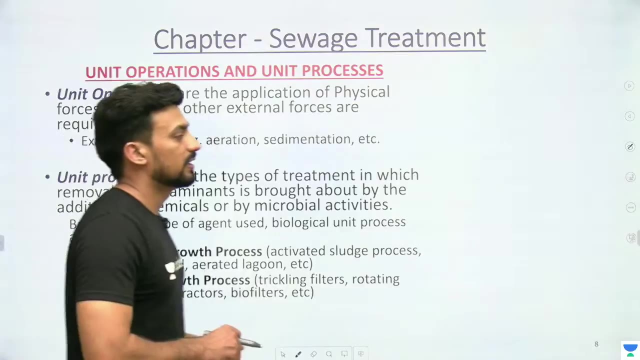 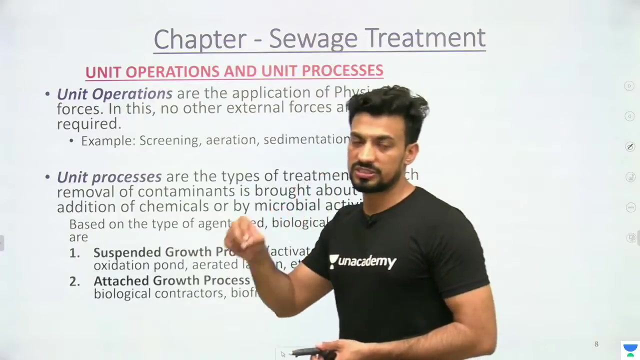 Thank you. If you have used chemical or microorganisms, then in such a case you will have what are called unit processes. Unit processes are of two types. first, suspended growth. second, attached growth process. To understand suspended growth, you can understand it as you make tea. then you put tea leaves in the pot of tea. you put tea leaves. 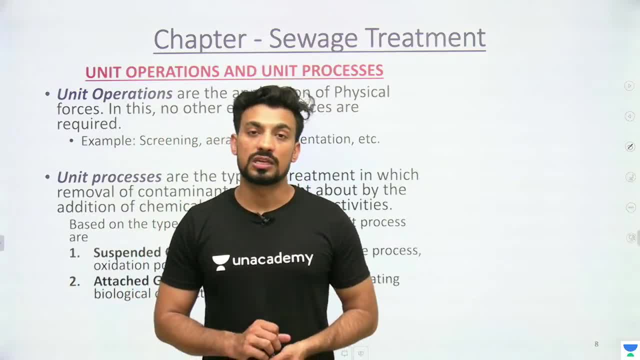 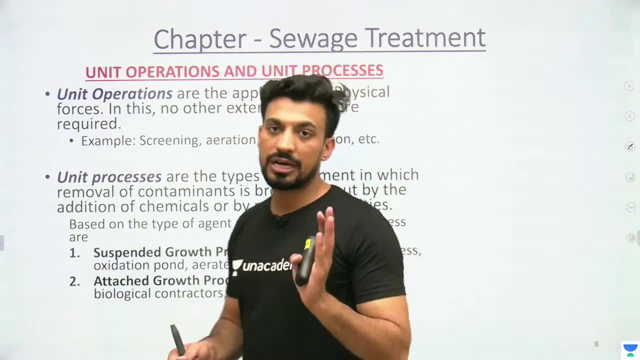 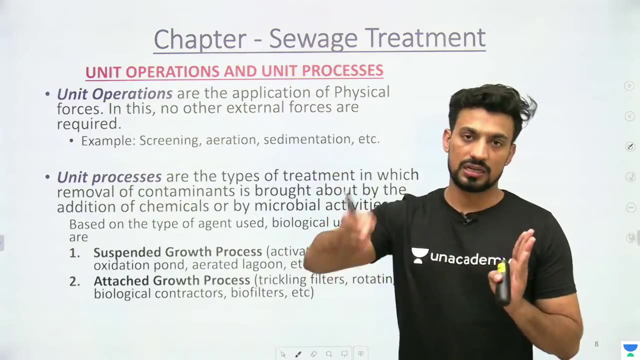 Now how it is in the form of that water. it is in its suspended form. it is suspended everywhere. Attaching means that you understand it as if you have a tea bag- The tea bags that come in these days. you become English, so keep the tea bag like this and pour hot water on it. 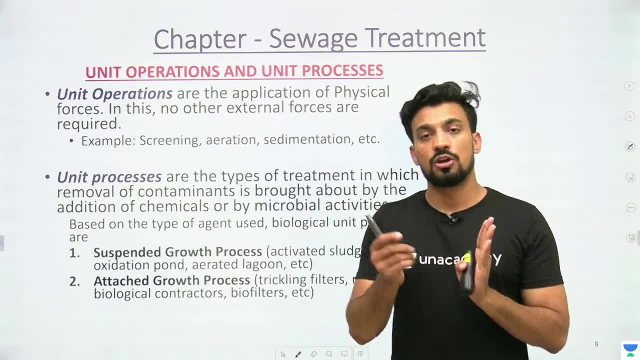 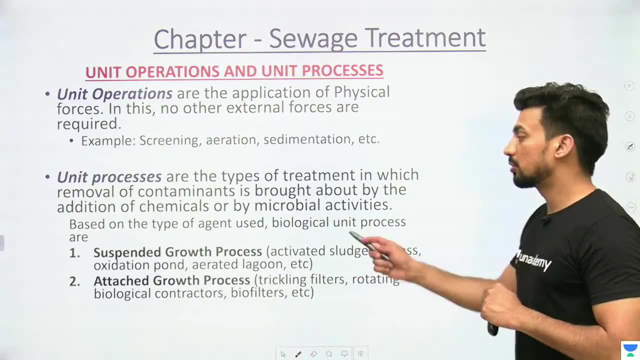 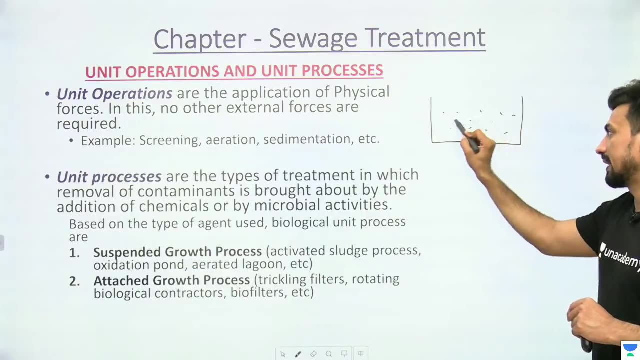 So that is an attached growth, that is, the tea is attached to that bag from that surface and the water is coming in contact with it and then going down here. So what happens in the suspended growth process? You have a tank and whatever microorganism is in it, the bacteria is in the suspended form in this water, that is, they are roaming around here and there in it. 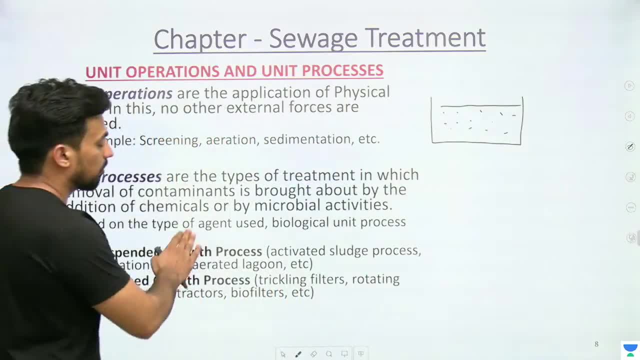 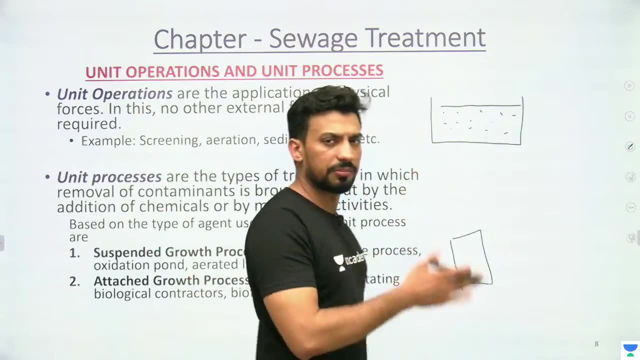 What has happened here? Suspended, it is in the form of suspension. What will happen in attached growth? Suppose it is on a wall, on a filter, on a surface, on a membrane. you have put bacteria on any layer And what are you doing? 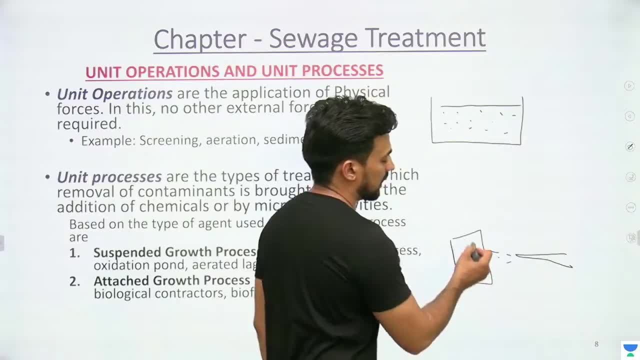 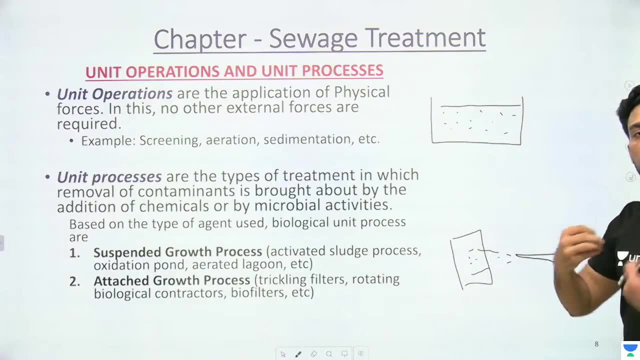 You have water on it, So because of which this water is coming in contact with that bacteria. So one thing happened: that in the whole medium, in the whole waste water- what did you do here? Bacteria is working in it to decompose the waste. 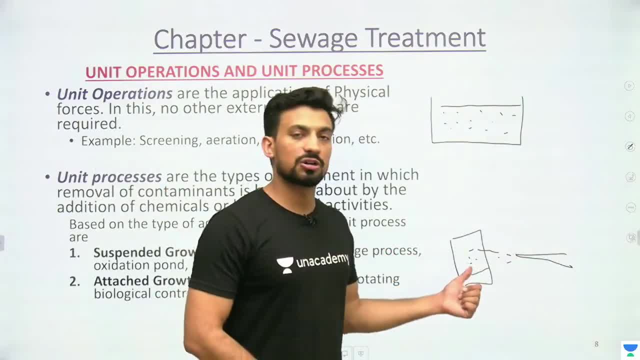 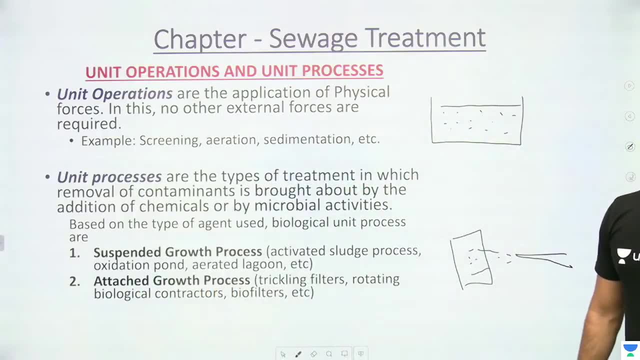 And the second thing is that we are bringing this waste water in contact with a surface. Bacteria is present on this surface which will decompose it here. Okay, so suspended growth is present in suspension. Attached growth means attached on a surface. 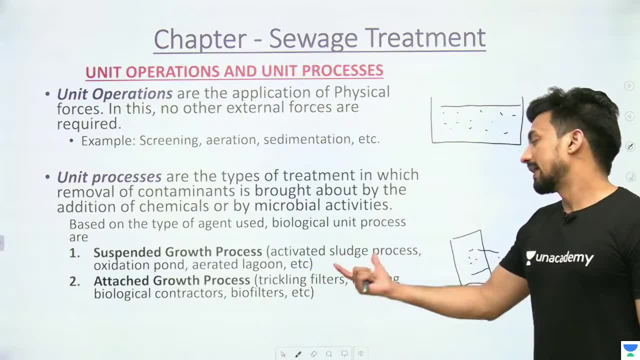 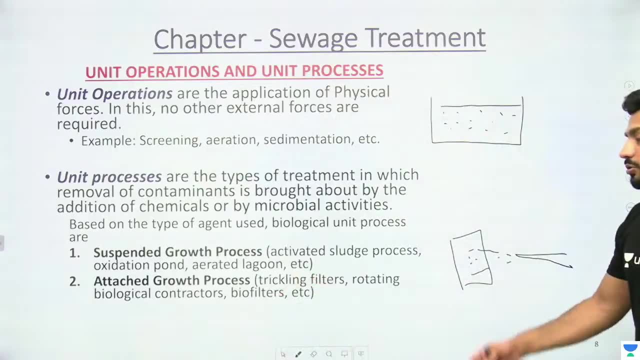 What will be the examples of suspended growth that we will read? Activated sludge process, oxidation pond, aerated lagoon, etc. If we talk about the attached growth process, then you will get trickling filters in it. Rotating biological contractors will come, biofilters will come. 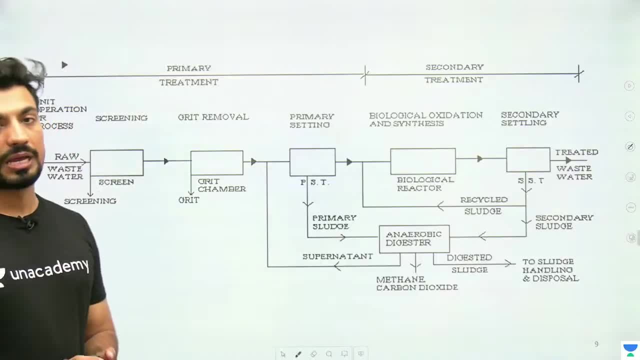 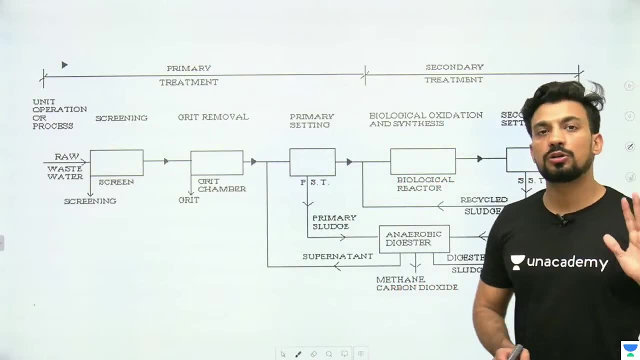 We will also read about them here, friends. For example, if we understand the whole process here, we have to see it once. we have to understand this diagram carefully, And after that this same thing will repeat again and again, This same thing will be read to these components, so you will keep understanding the whole process. 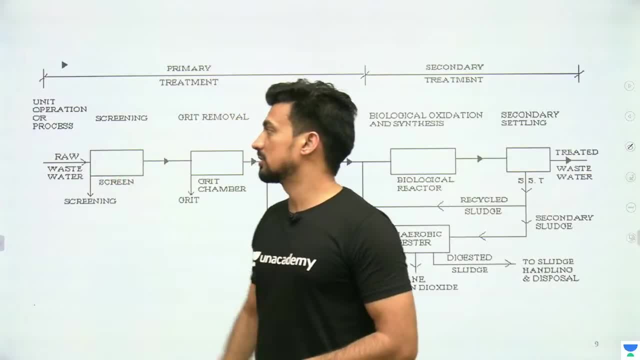 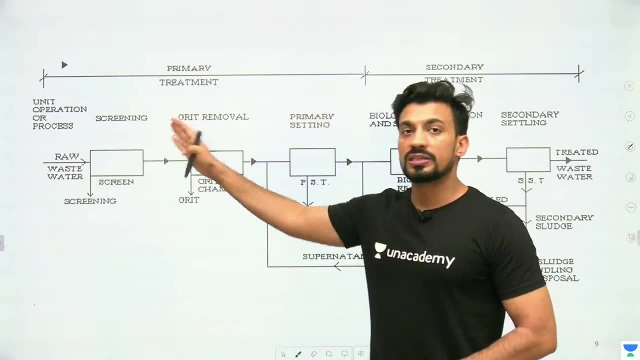 The first thing is unit operations or the unit process that you have. If we talk about unit operations, which of these unit processes have started from here? Screening, grit removal, primary settling, biological oxidation and synthesis, secondary settling, etc. etc. 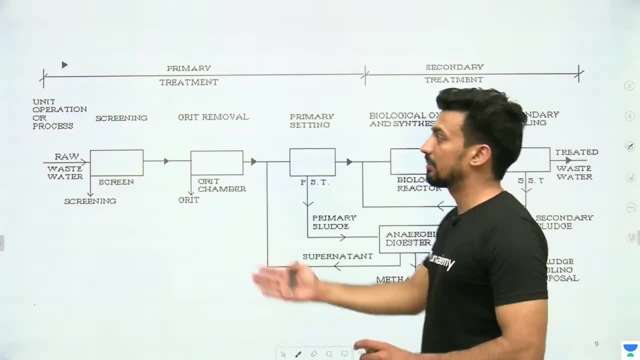 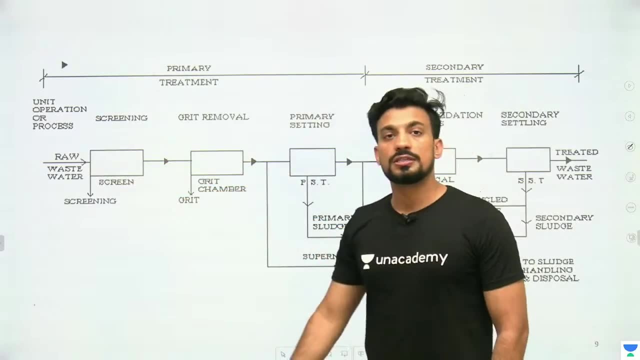 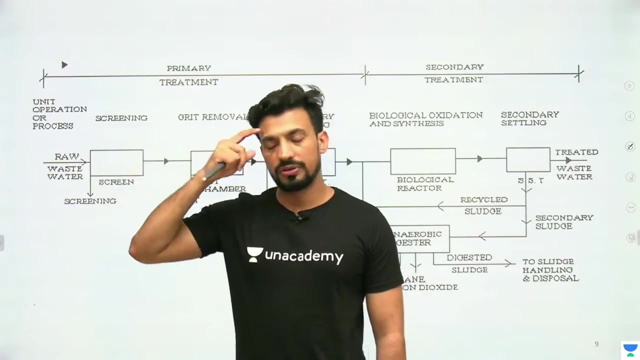 All these operations or processes have been told to you about them here, So you have given the names of the unit operations or processes here. Now let's see what happened to the process. First of all, raw water came. Raw water or sorry, waste water. 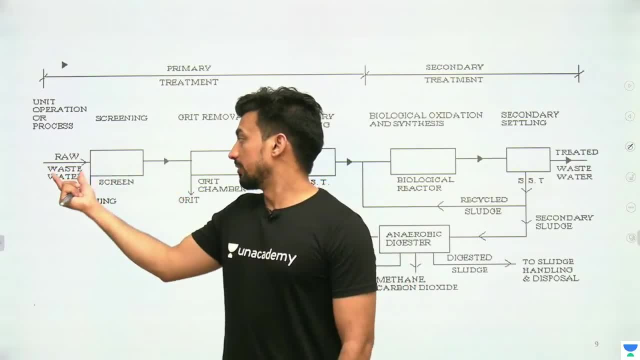 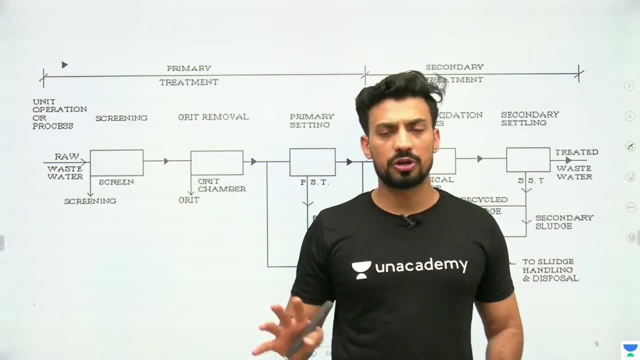 Such water that you have not treated. So waste water came, let's call it raw waste water. Screens were attached So due to the application of the screen, the large impurities in the waste water, the big garbage, was separated from here. 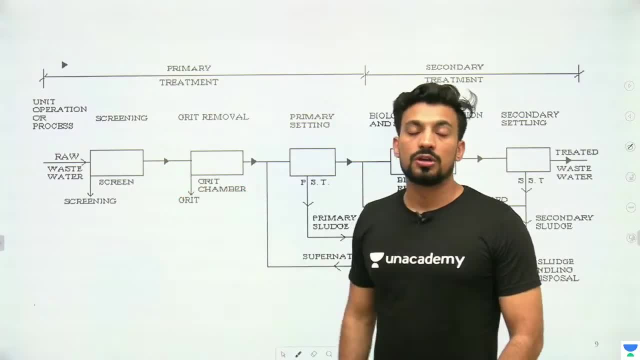 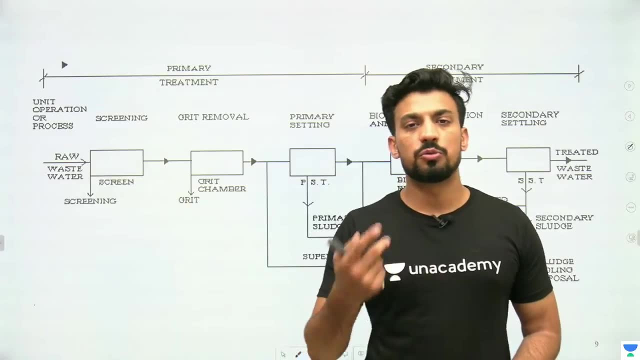 After that, what happened? The waste water went ahead. If we talk about the floating material of the screen, then what can you imagine in the waste water? Some plastic bottles must also be coming in it. Some dead and decayed animals or plants must also be coming in it. 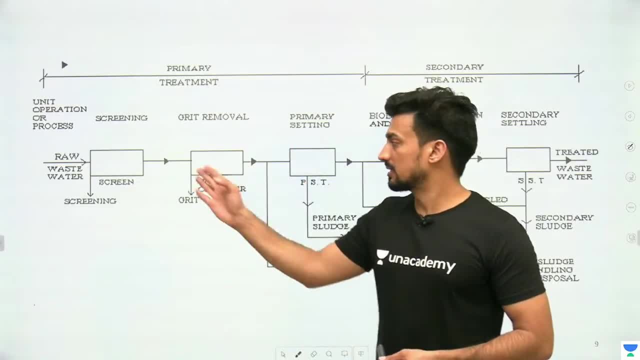 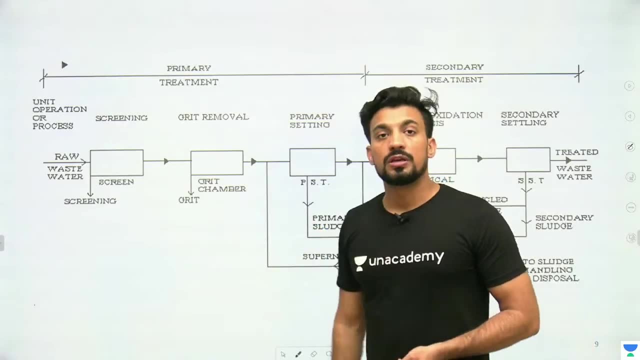 And all the big waste must be coming. So here, the screens separated them, They separated the floating material. Then, after that, friends, you came to the grit chamber. If we talk about the grit chamber, then what will the grit chamber do? 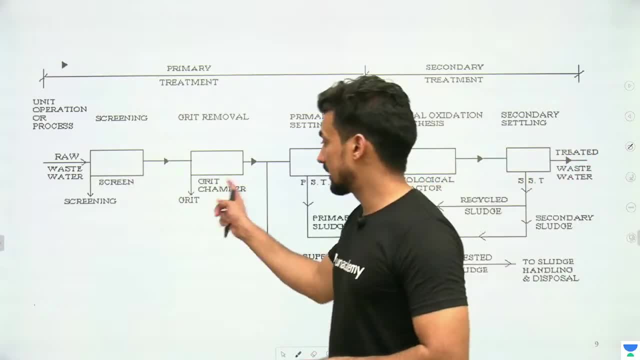 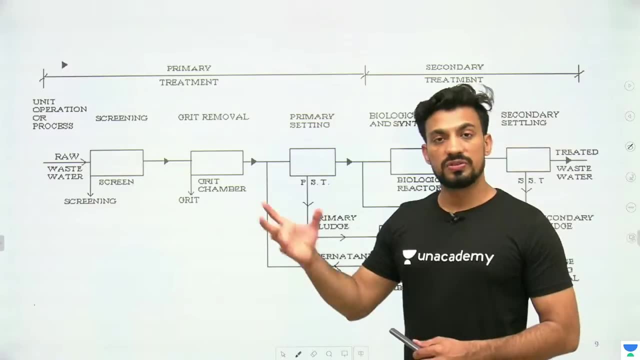 It will remove the concrete stone. Those who have more weight will be removed from here. The grit will be removed. Now what do we understand by concrete stone? Inorganic? What will happen to the inorganic waste? What will it do to the inorganic content in the waste water? 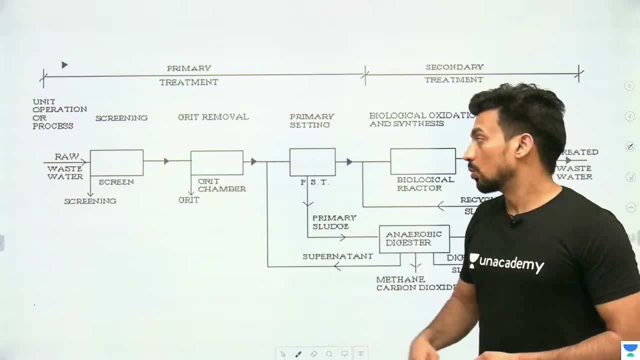 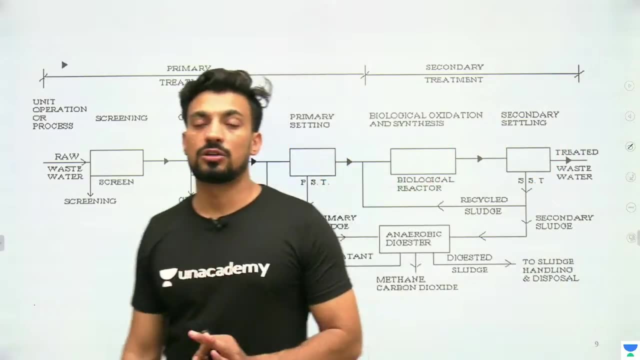 It will remove it Here. the grit chamber will be removed. After that, this waste will go to the primary sedimentation tank. The name itself makes sense. There has to be sedimentation Due to the action of gravity, Particles will settle here. 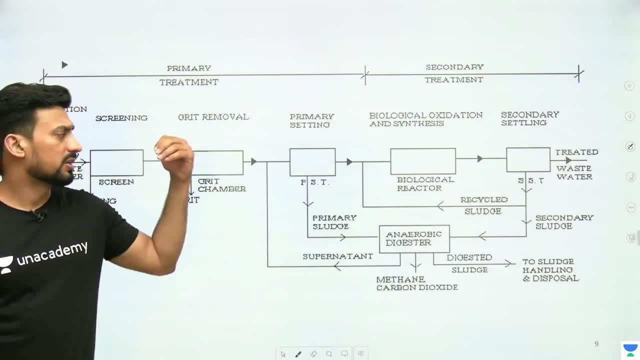 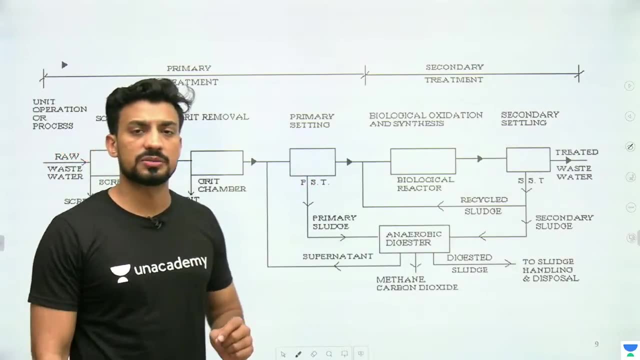 So here whatever inorganic is left, of a very small size Or organic Majorly. here organic is removed by 60%, It will settle. Now what do you understand by organic waste? What does organic waste mean? It means particles of very small sizes. 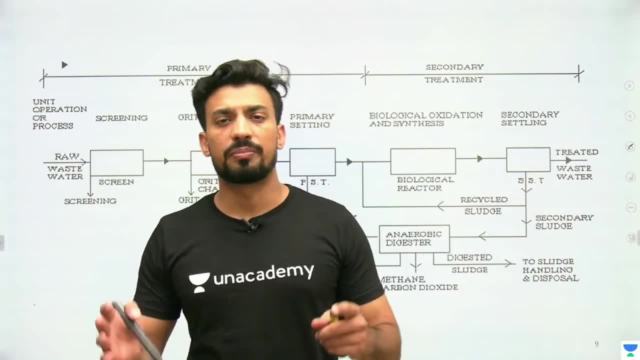 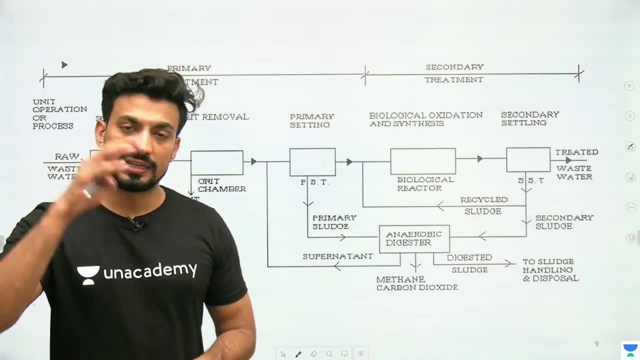 Whatever you have, If there are vegetables, If there are any plants, If there are animals, The smallest particles of these, The smallest organic components Which are not settling, Which are not settling in the primary sedimentation tank, What will we do? 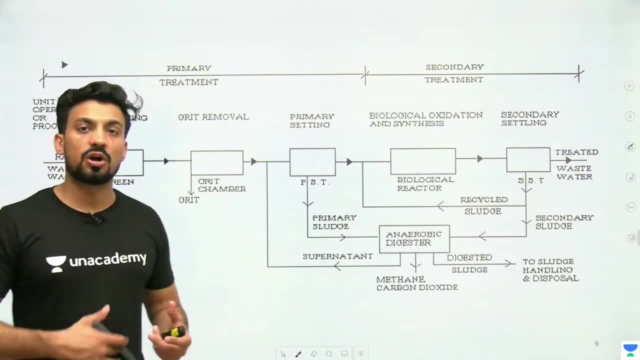 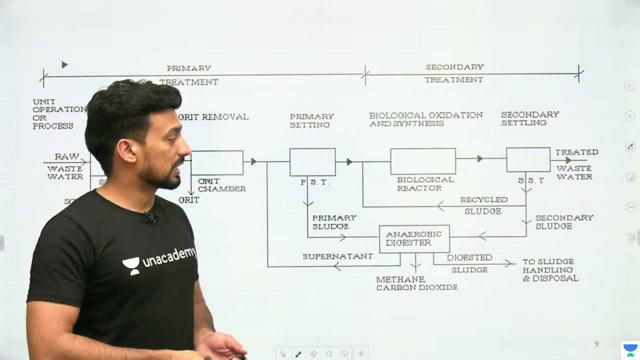 We will bring them in the contact of oxygen. We will bring them in the contact of oxygen, We will bring them in the contact of bacteria So that they decompose it, And then what happens after that Settles. So then they will be sent. 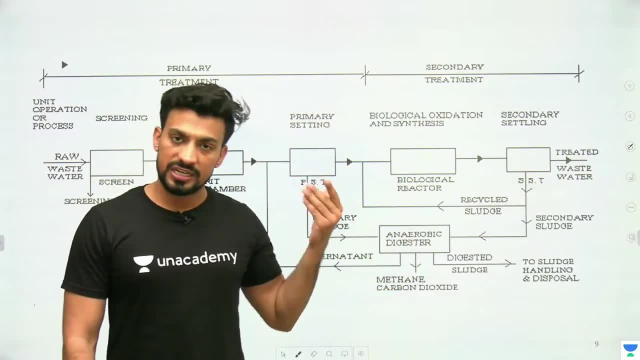 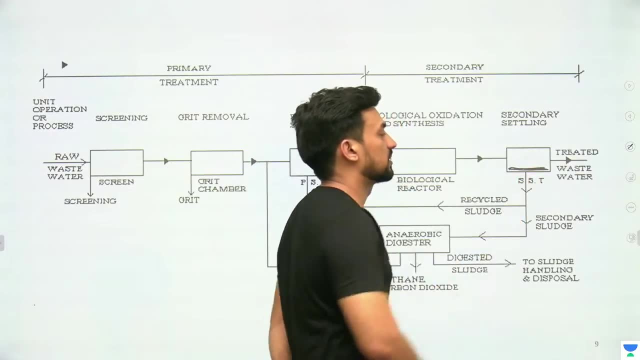 In which, In the secondary sedimentation tank. What will happen after going to the secondary sedimentation tank Now, when the bacteria decomposes it? Then it will settle down here. Okay, It will become sludge. When it becomes sludge, 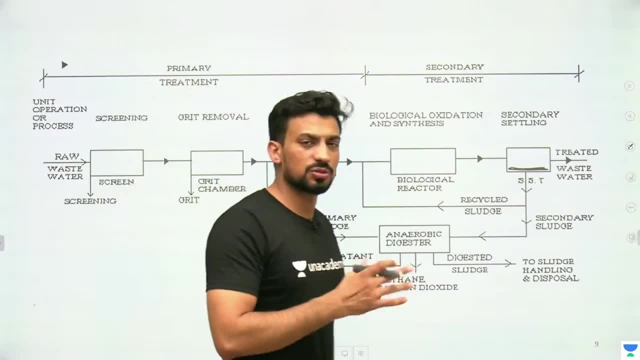 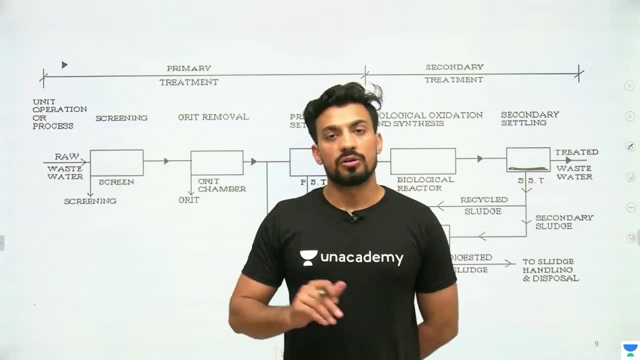 That solid is separated. The solid is separated from the water, So now It's not like it's completely pure water, But the solid particles, The organic particles, The inorganic ones got stuck here. The organic ones that were left, The small sized ones. 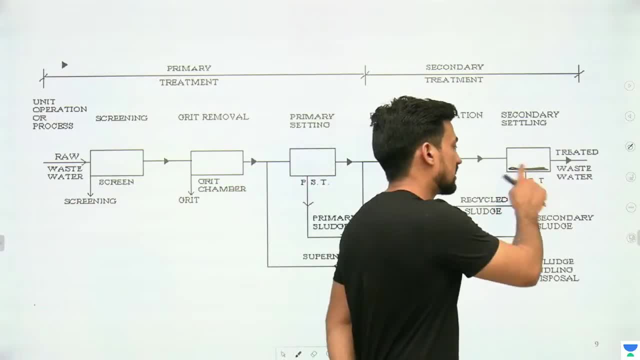 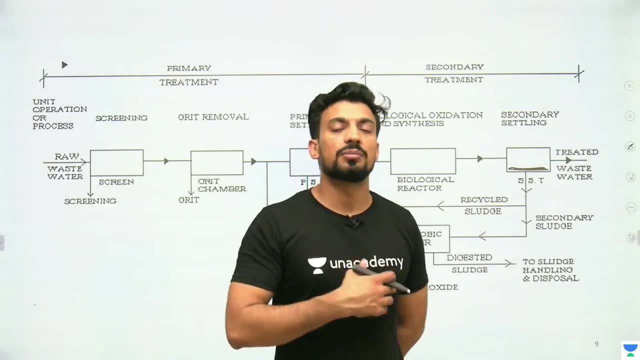 The floating ones. What did they do Here? They got stuck in the form of sludge And, from above, The treated water. We will not call it clear water, Treated wastewater Which we can take to the rivers Or to such places. 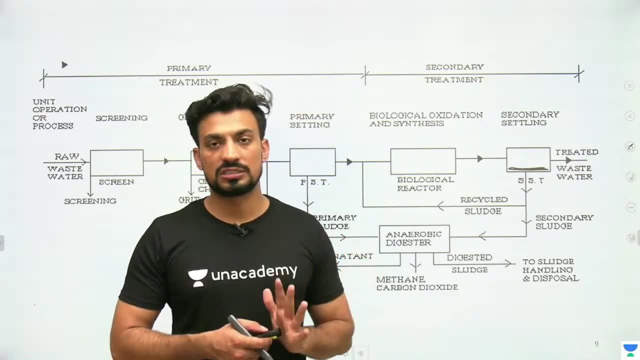 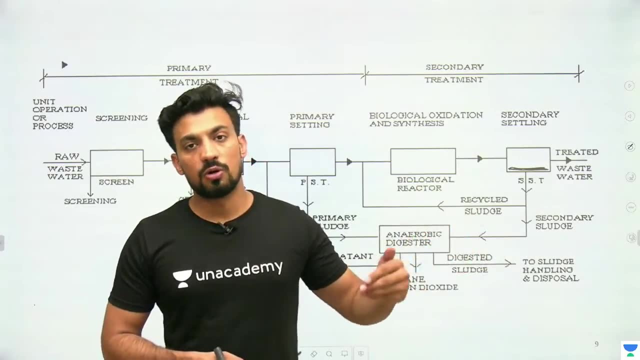 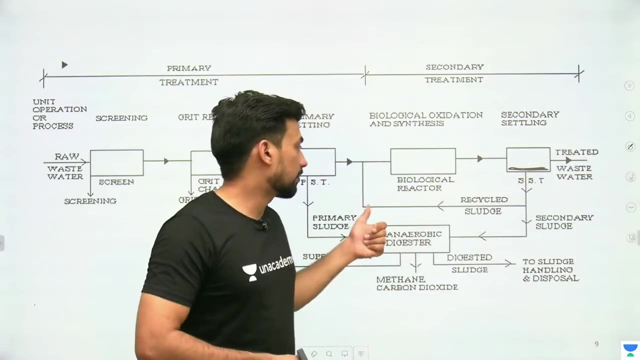 Where Further further It will be purified And it will not harm the environment. So if the wastewater was sent along with the organic waste, Then it would have polluted our environment. So what did we do to it Through this process? Now, what do you see this process coming back? 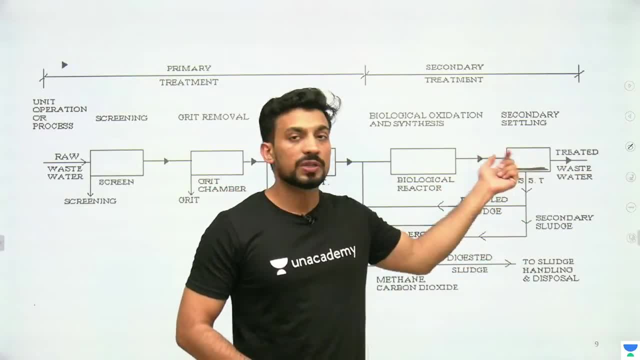 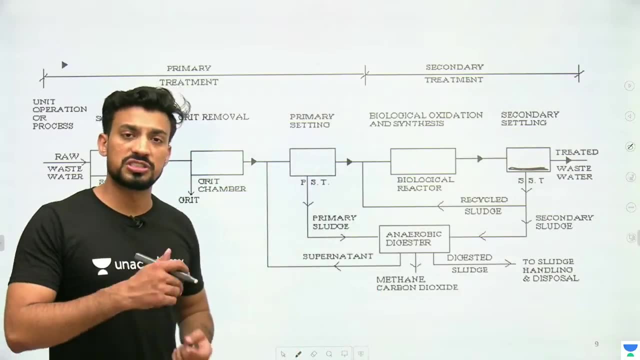 This process is coming back. It is visible that this sludge form, Whatever aeration was done from here. You introduced air Means, gave a lot of oxygen To this wastewater, So that the waste decomposes Now in the presence of bacteria. 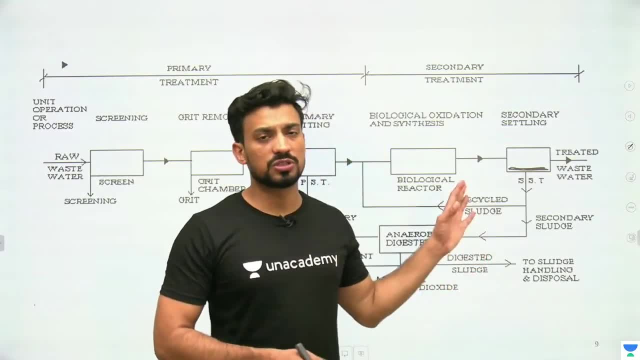 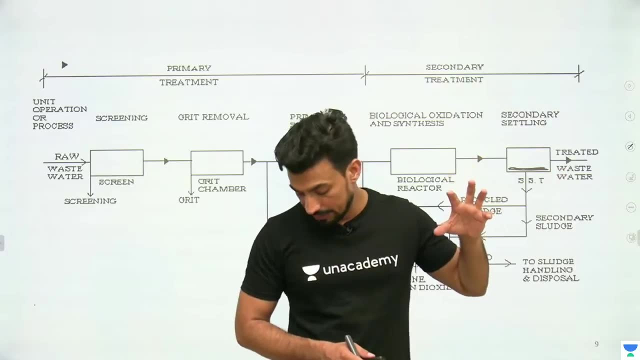 The bacteria needs oxygen, Or the bacteria is decomposing the waste here. So when it decomposes And here the sludge forms, So what happens? in this sludge A lot of bacteria will be present And we can use that bacteria. 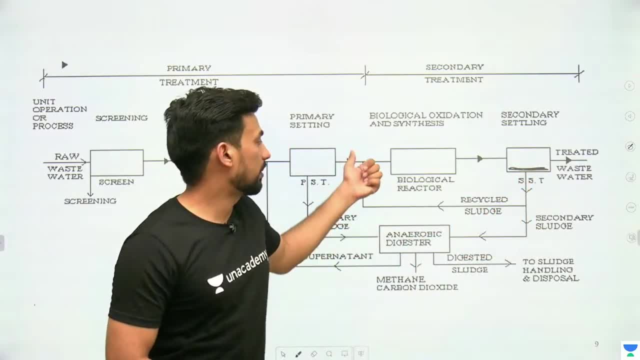 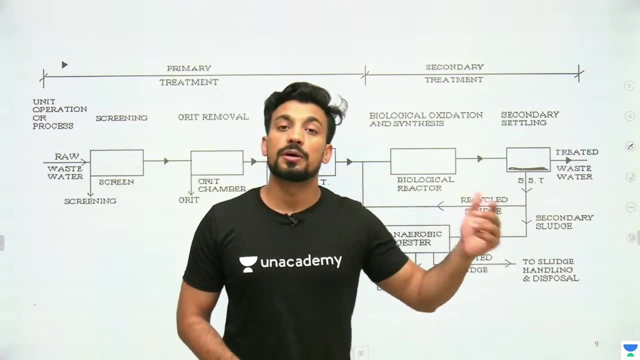 We picked up this bacteria from here And bring it here and add it back, So that the further wastewater that is coming now When it goes into the biological reactor, Then more bacteria will be present in it- Or this recycling, Or this recycled sludge. 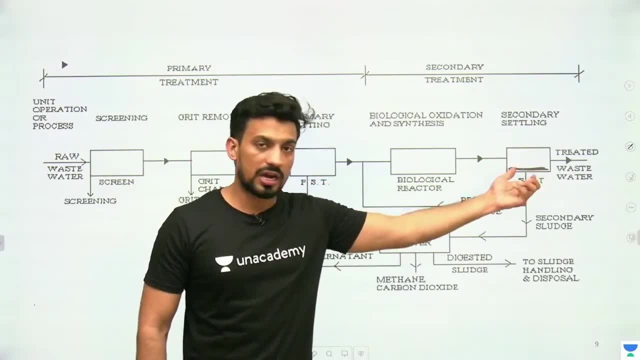 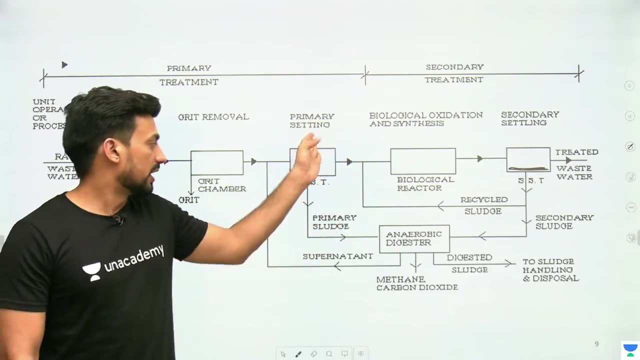 Put it in the primary sedimentation tank. You pick it up from the last, Take something out of it And bring it here and put it So that when the water came in the primary sedimentation tank, Then a lot of work will be done here. 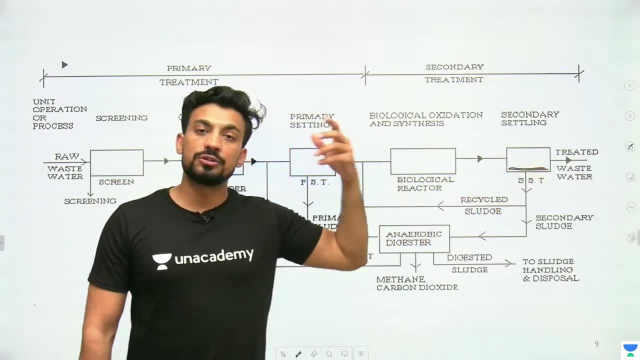 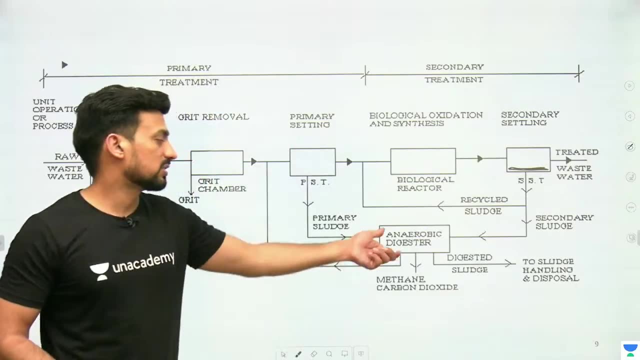 Or from here to here. When that water reaches, Then bacteria has already decomposed that waste in it And our process will be faster here. So we can do this. If we talk about the absence of oxygen here, Then you can also put it in anaerobic digester. 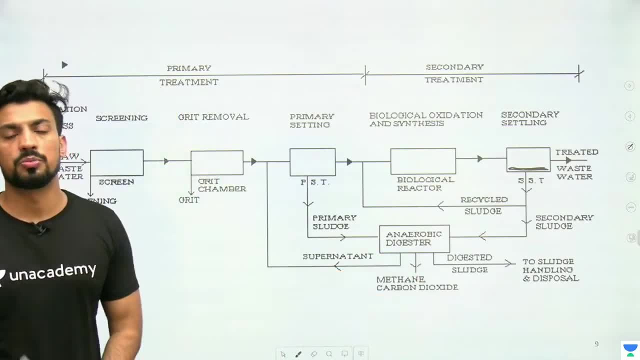 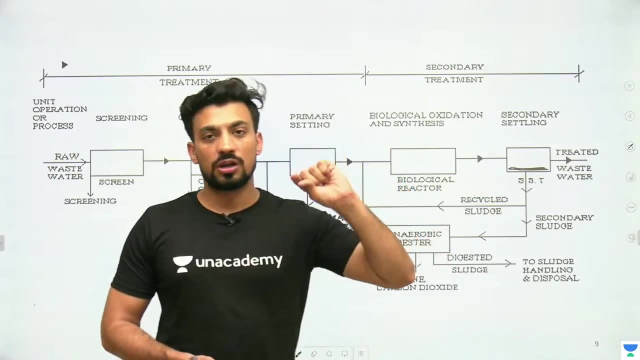 And from here you will also get methane or carbon dioxide In anaerobic reactions. The sludge that will come out, The completely settled portion, The completely solid portion, This portion will come out. How do you have to handle the sludge further? 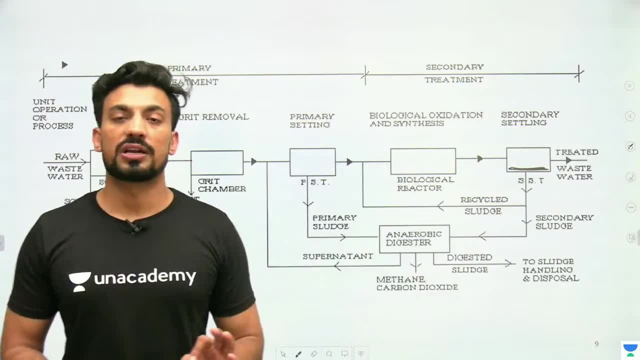 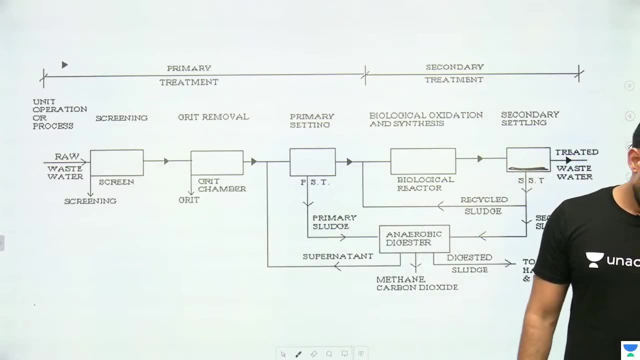 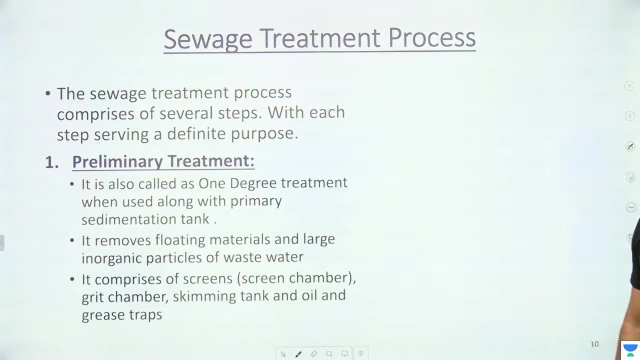 What to do with it. Do you have to use it in agriculture Or where to dispose of it? You can use them Overall. the whole process will go on like this again and again. So let's understand one by one. This was just an overall idea that what we will study. 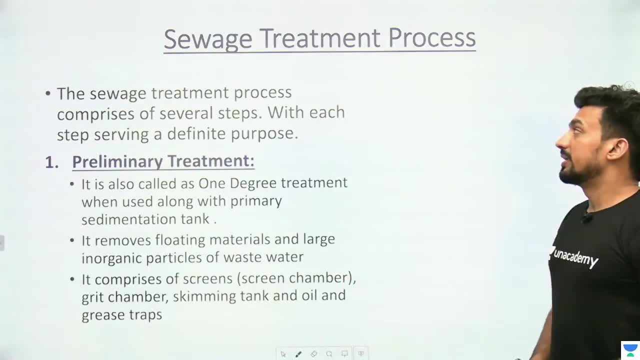 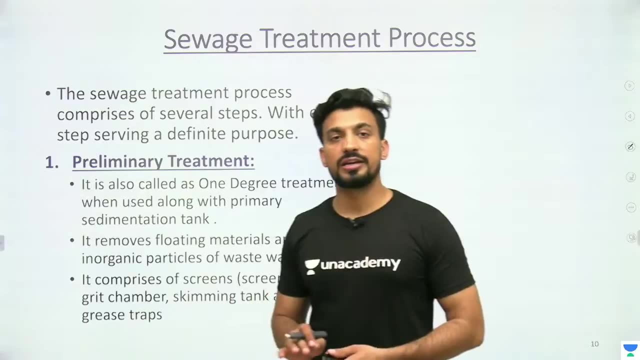 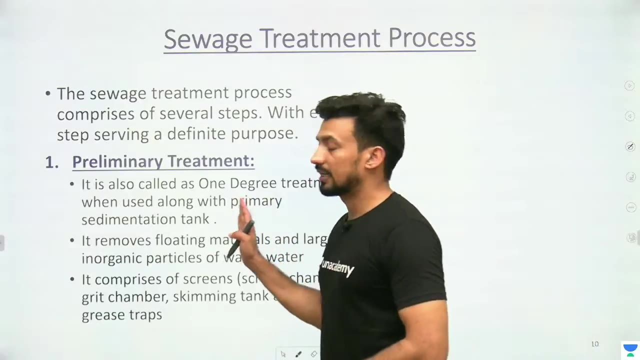 And now let's start here If we talk about sewage treatment processes. So what are the steps in the sewage treatment process? The first is preliminary treatment, Preliminary treatment, or one degree treatment, We call it. How far does the process come in one degree treatment? 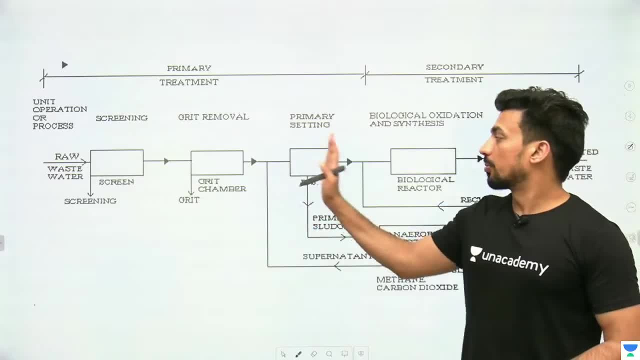 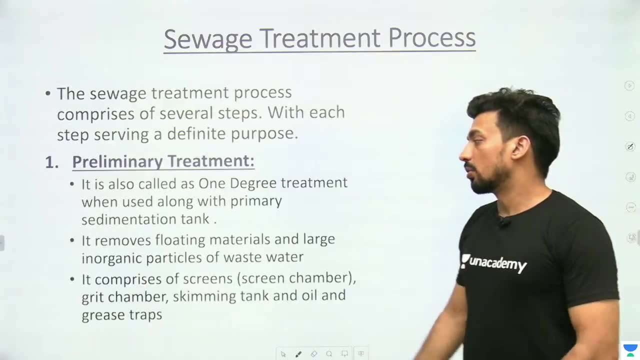 The process comes up to the primary sedimentation tank. Whatever we have studied So up to the primary sedimentation tank. What do we call it? Preliminary or primary treatment? It remains up to here. So it removes floating material. Where does floating material come? 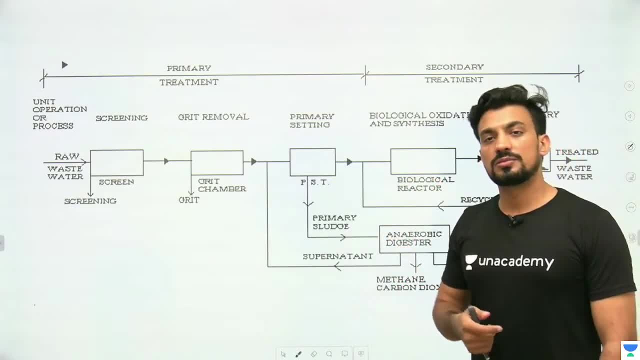 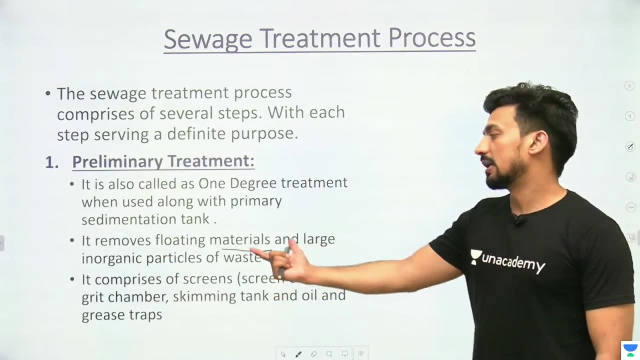 Now see this: Say the good thing about this chapter And say the bad thing too. The same thing will come again and again, That we have already understood: Floating material came from here, Moved here, So we wrote it. It removes floating material. 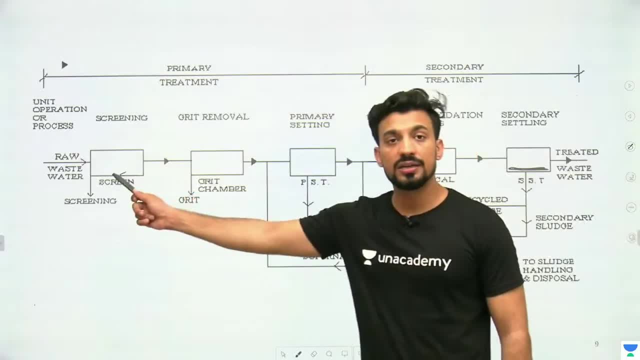 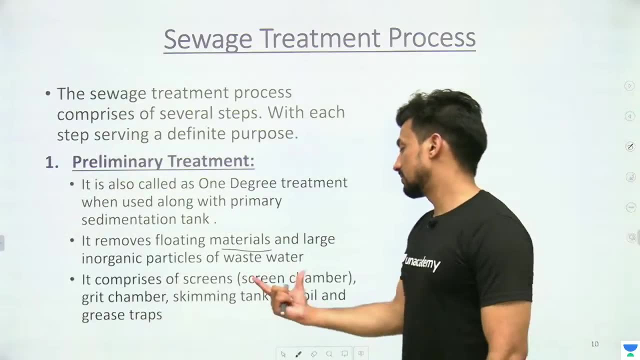 And large inorganic particles. Floating material comes here- Inorganic particles. Inorganic particles Will be removed in the grit chamber. Here. the stones will be removed here. It comprises of screens. There will be a screen here. There will be a grit chamber. 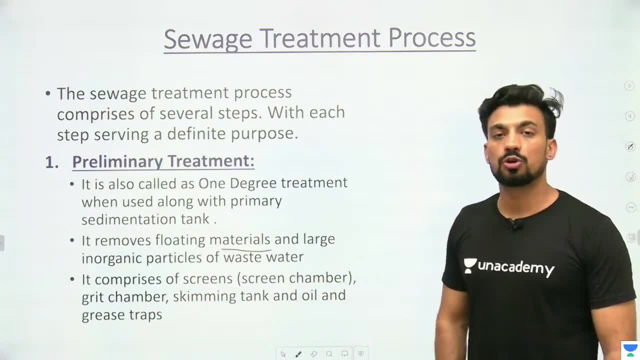 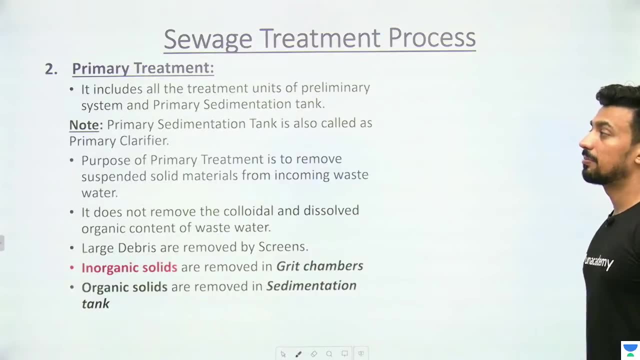 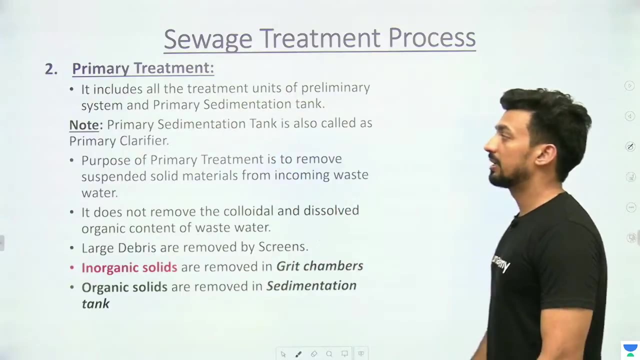 Skimming tank, Whatever you have here. There is oil, There is grease To remove them, Skimming tank And you use your oil grease traps. Then, after that, friends, Let's talk about primary treatment. So in primary treatment It includes all the treatment units of preliminary system. 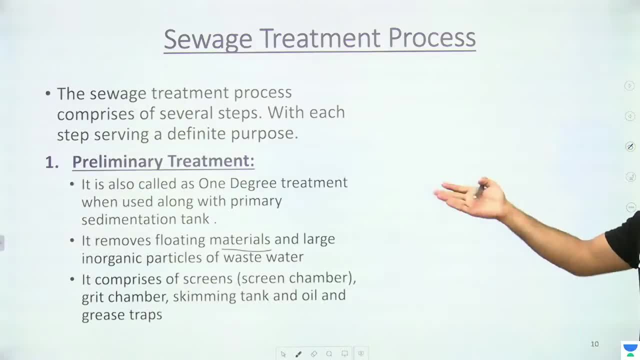 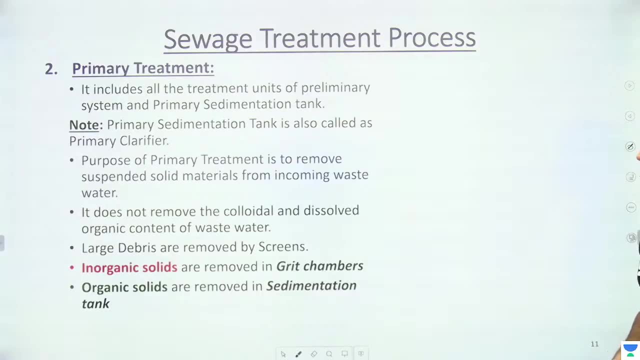 And primary sedimentation tank. So here it is the same thing. If we talk about preliminary or primary, Then the process up to primary sedimentation tank We include that here. Primary sedimentation tank is also called as primary clarifier, Primary clarifier. 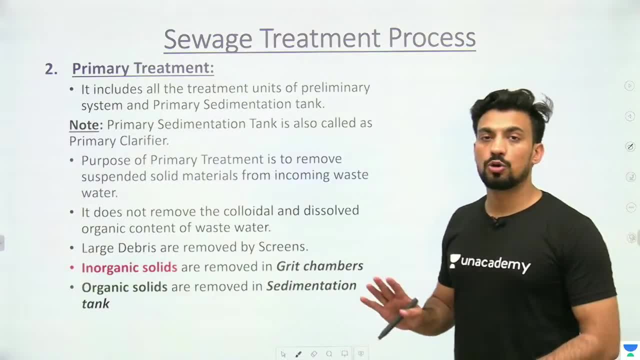 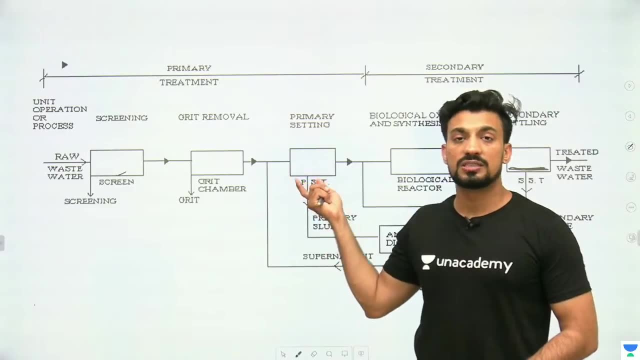 We will call the primary sedimentation tank, Where we have not used any biological reactor before that. After the grit chamber, What we did directly Here, we sent it to the primary sedimentation tank, Where about 60% of the organic particles will be settled. 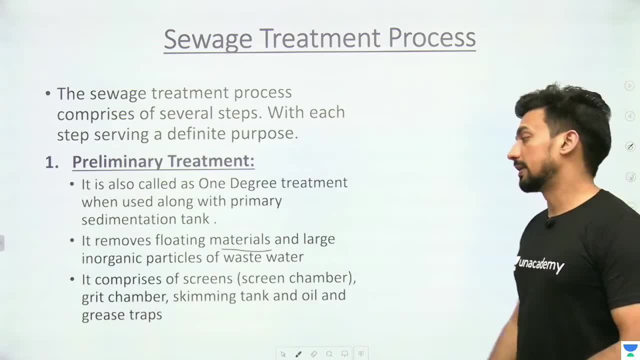 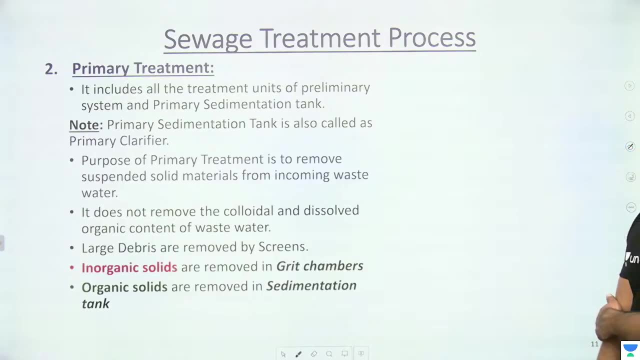 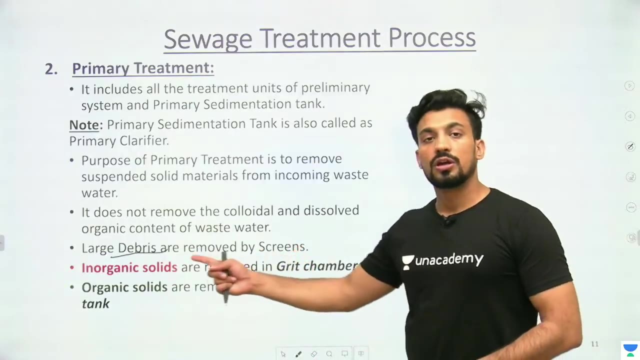 Which will be saved. We will send further processes to them Here. It does not remove the colloidal and dissolved organic content of waste water, So the big debris will be The big garbage That will remove the screen. Inorganic solid. 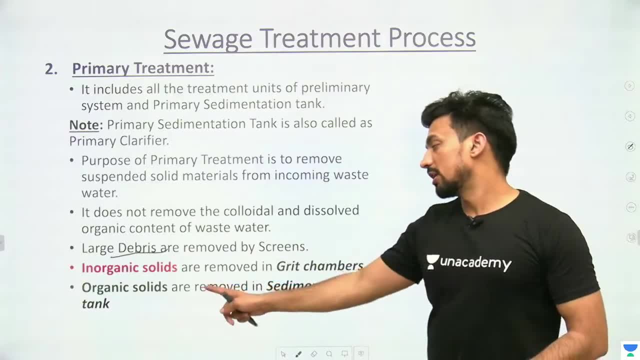 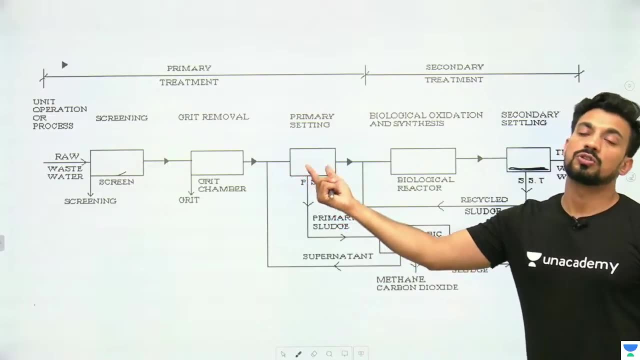 Or the grit will be removed in the grit chamber. Organic solid will be removed in the sedimentation tank. This sedimentation tank, If we talk about primary, So it will be removed here to a large extent, The small ones Which are not settling. 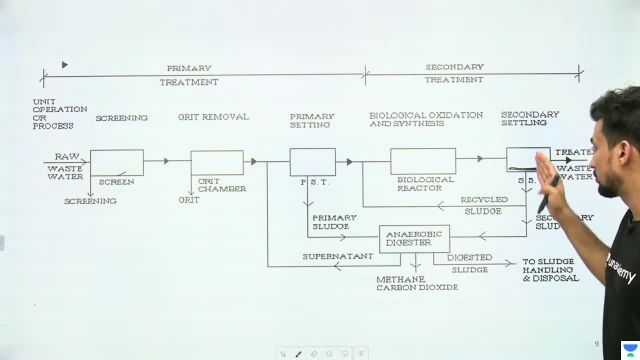 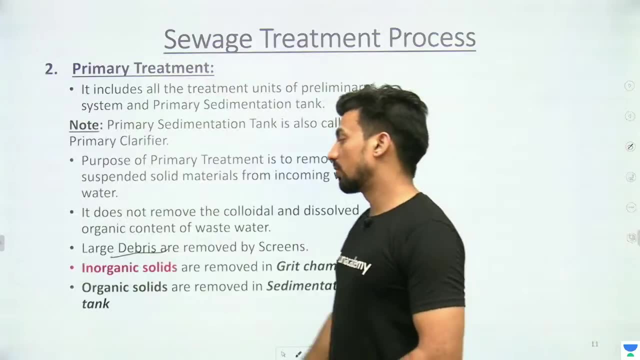 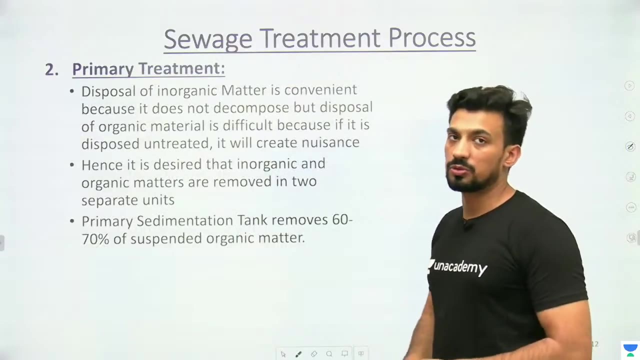 They are in the biological reactor, Bacteria will decompose them Then. after that It will settle down in the secondary sedimentation tank In the form of sludge. So you have this overall overview of it In primary treatment. Here also we are talking about the process up to the primary sedimentation tank. 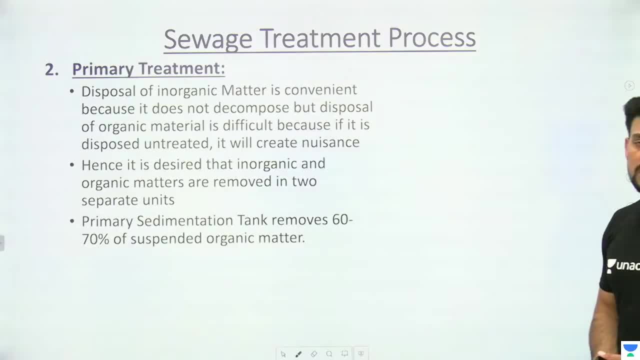 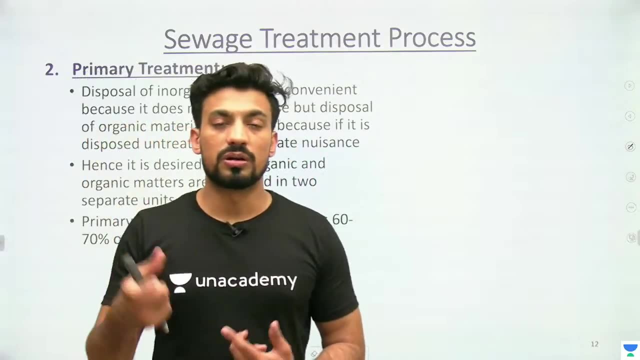 Disposal of inorganic matter is convenient. You have a simple thing: When you sweep in your house, So you sweep Whatever you sweep. So when you sweep in the house, When you sweep in the house, So what is the dust? 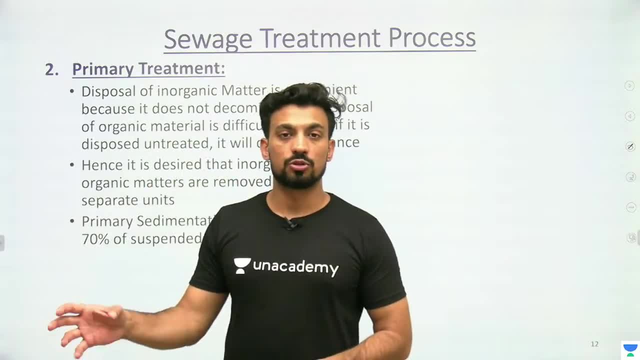 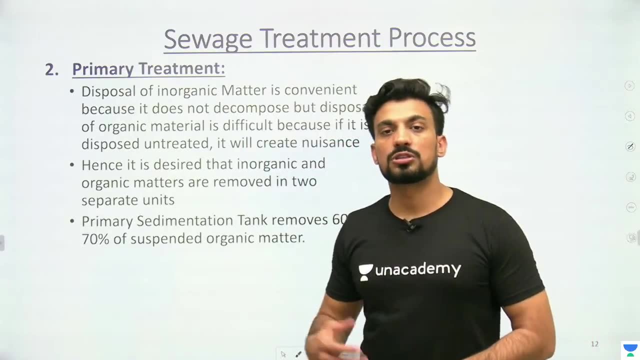 What is that? It is inorganic If there is dust somewhere, So it is not creating any smell. So whatever stones are inorganic particles. Those inorganic particles do not harm the environment so much. They will not create any bad smell. 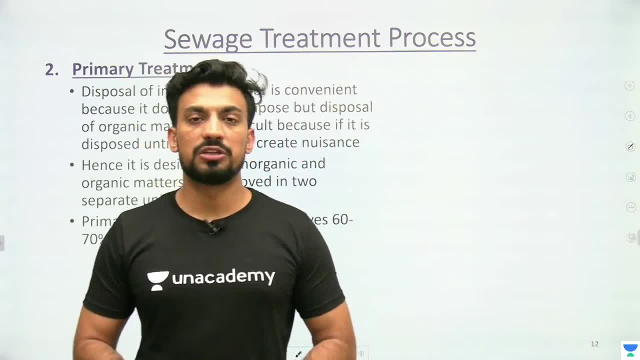 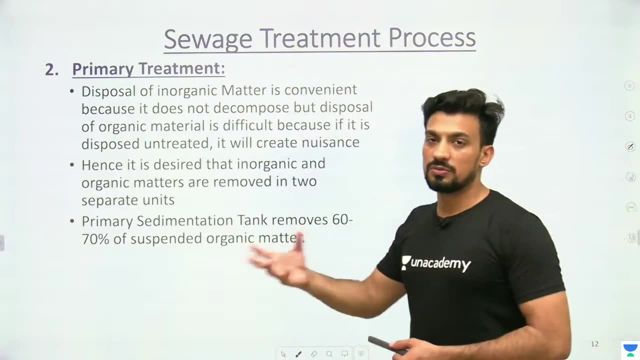 Because of them, bacteria does not spread, Fly does not spread. Diseases will not spread Because of them, Because of inorganic people, But organic matter, Any organic matter You dustbin, Which is in your dustbin, Whatever is the waste of the kitchen. 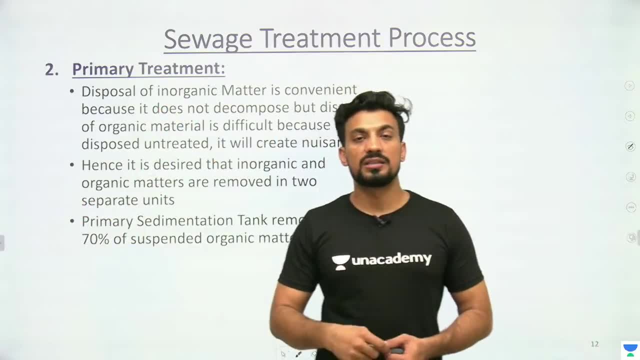 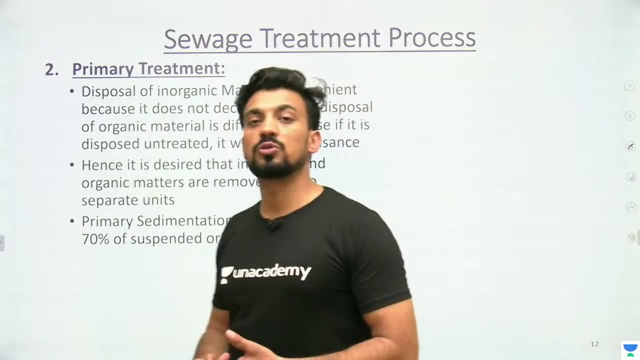 The peels of vegetables, The peels of vegetables. Leave it for 2-4 days And you see What will happen in the whole house Because of that. So organic matter Which rots, Which decomposes, It is more important to handle. 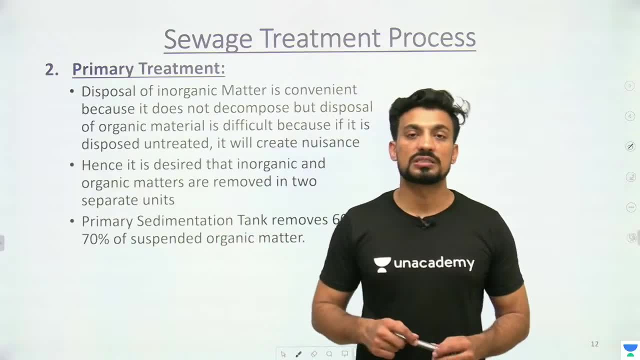 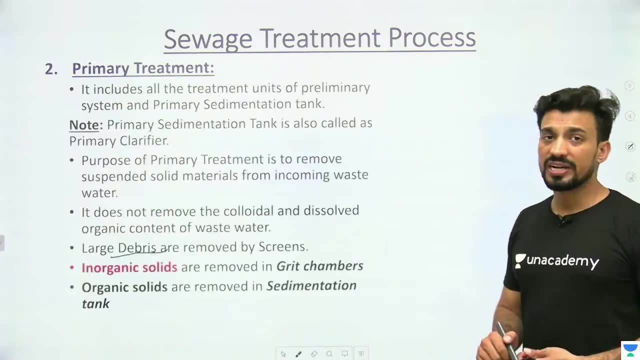 Inorganic If you remove the pebbles And you can dispose of it easily. So handling organic is very important And if Grid chamber is not installed, If grid chamber is not installed, You will say We put it in the primary sedimentation tank. 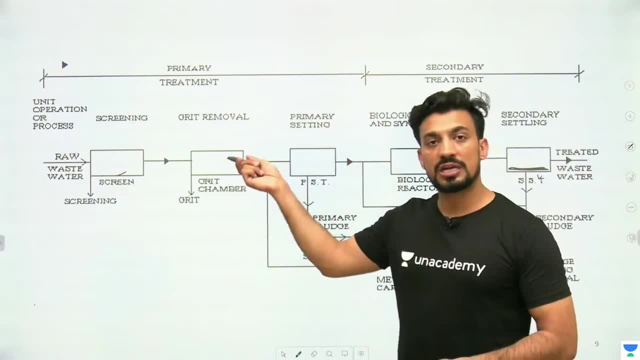 Why do you have to spend the grid chamber here, The particles of the grid chamber, Instead of settling here? Come here and settle. It has to settle. We have already made this tank. You are here, But if you do this, Then inorganic and organic. 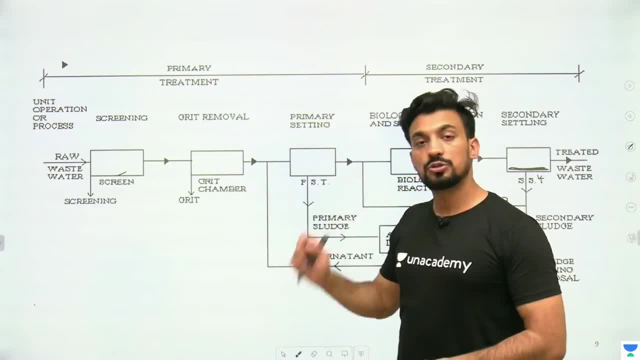 Both will be mixed, And if both are mixed Then it is more difficult to handle them. If both types of particles are mixed, Then it will be more difficult to handle them. That's why we say In the grid chamber: Remove the inorganic first. 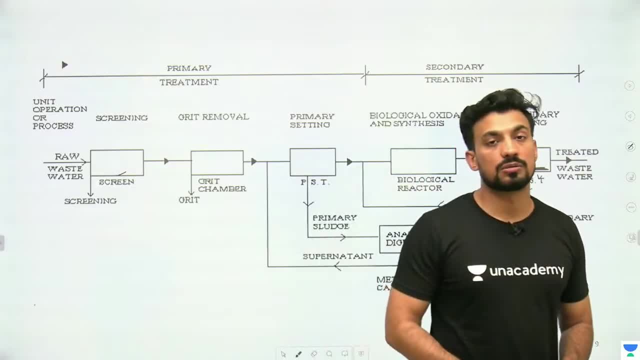 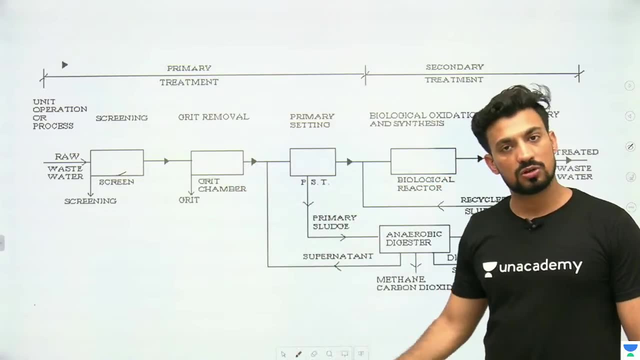 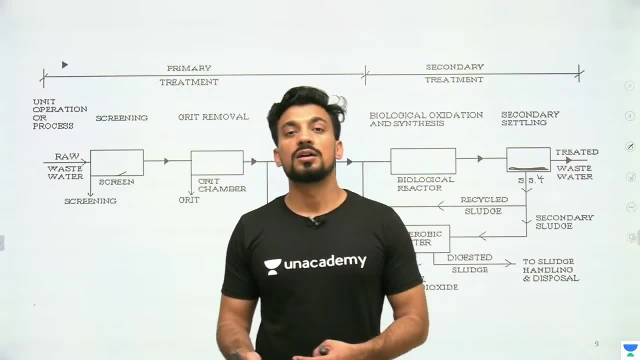 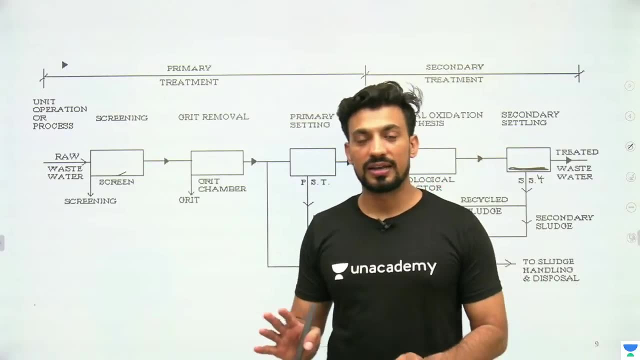 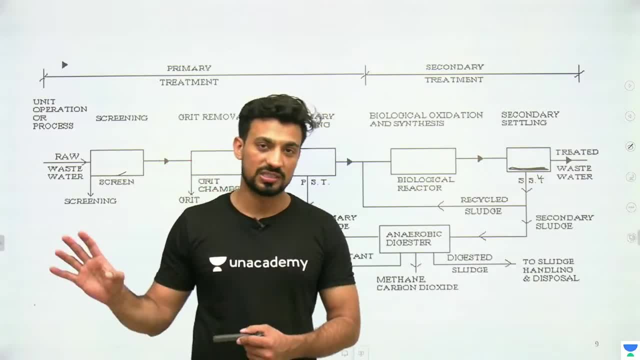 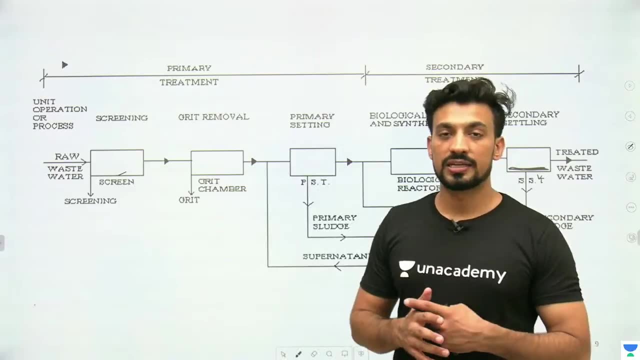 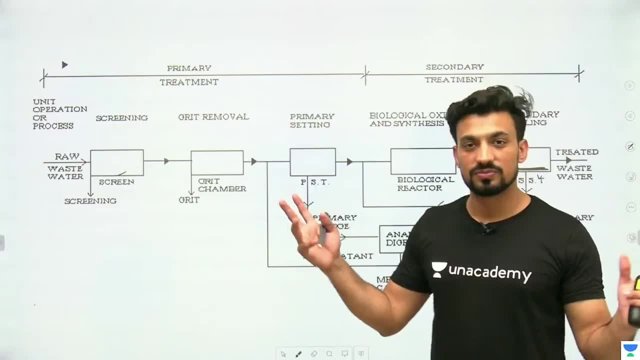 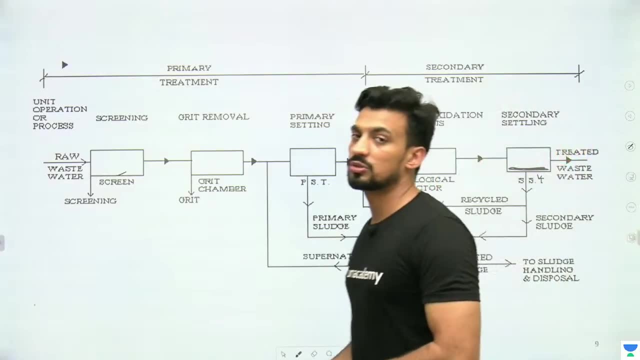 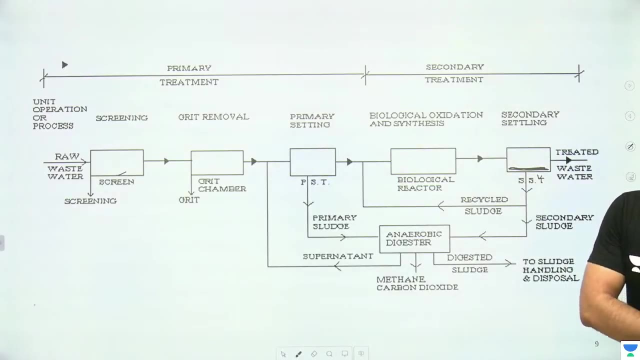 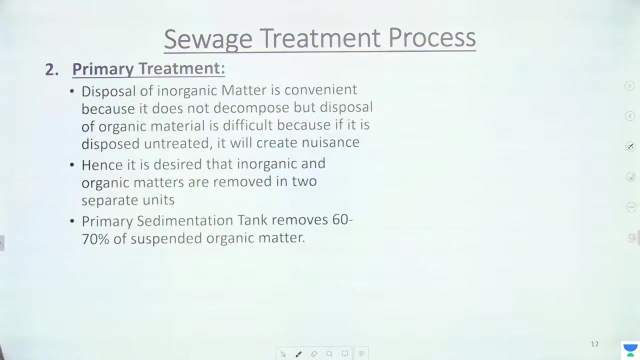 Inorganic, Inorganic, Inorganic, Inorganic, Inorganic. So organic waste is decomposed. bacteria decomposes it, so that's why it is very important to handle it. Okay, who eats these fruits in Austin? Let's move ahead. there are very basic things here. 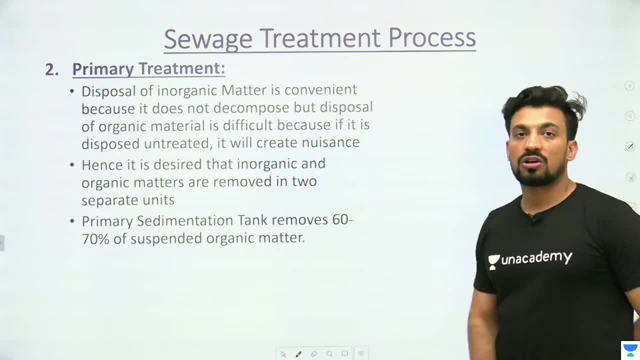 In primary treatment we say to remove inorganic and organic separately. So don't do this to save the cost of the grit chamber. let it go to the primary sedimentation tank. Now why are you repeating the story again and again so that you remember that in the grit chamber inorganic is removed? 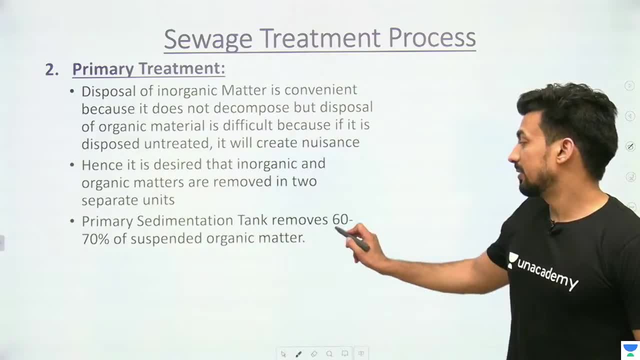 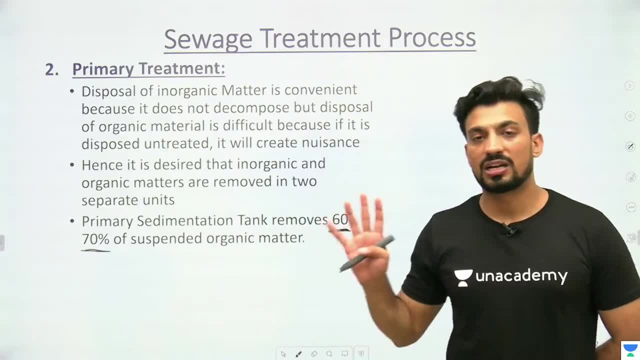 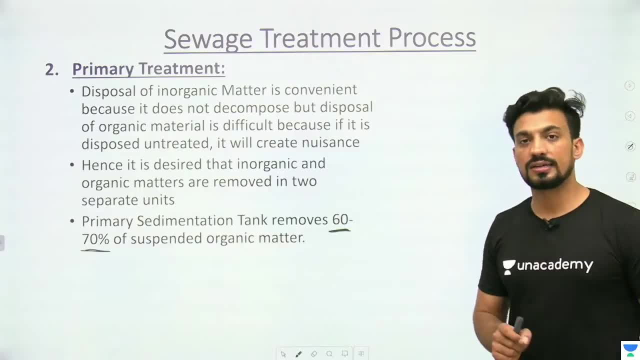 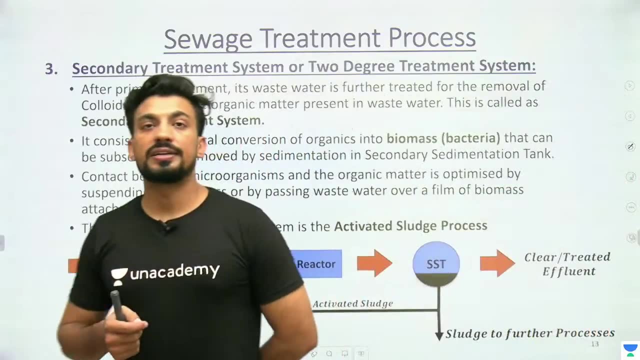 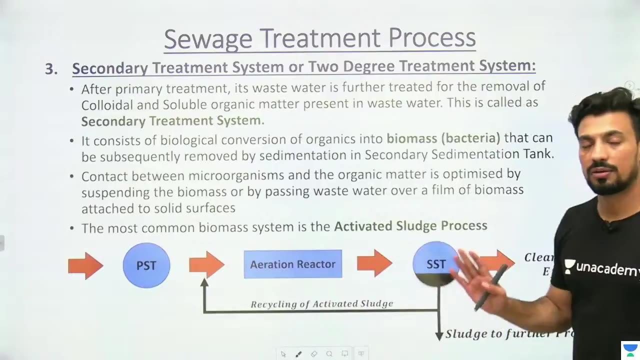 But then some of those particles that are not getting settled, which will need to be settled for our next process. So now let's talk about secondary treatment, or now second degree. First you can say preliminary, primary, that was the primary sedimentation tank. 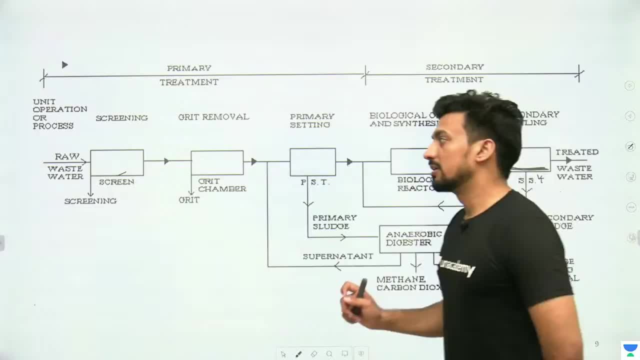 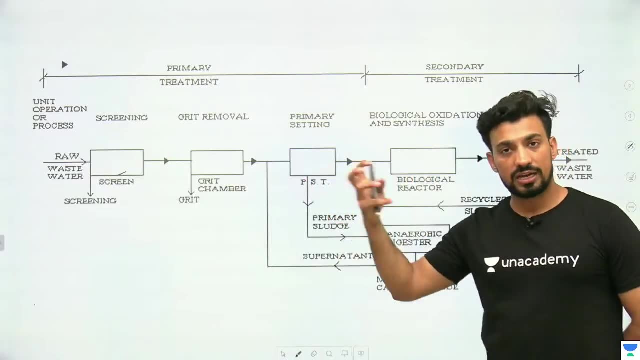 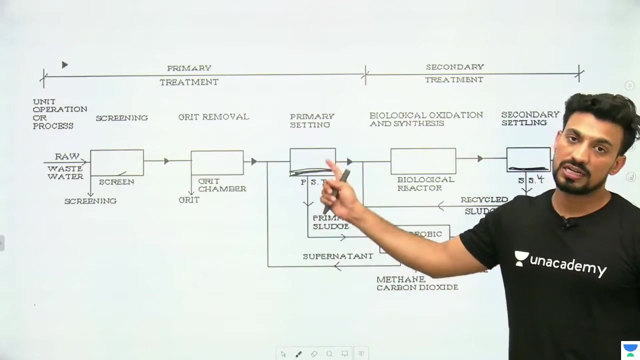 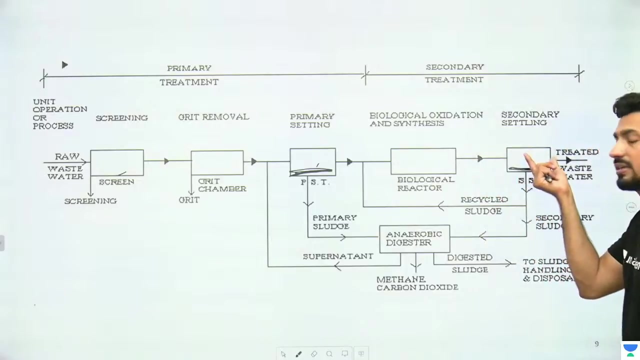 Now you understand the whole story. it will go on like this again and again. the floating material was removed from the screen, then the concrete stone was removed, the inorganic particles were removed in the grit chamber, then the organic particles came in the waste. so 60-70% of the particles settled here and they were separated, but some that were not settling, they were sent ahead. they were decomposed with oxygen and bacteria in the biological reactor and then they went to the secondary sedimentation tank and now they settled here in the form of sludge. 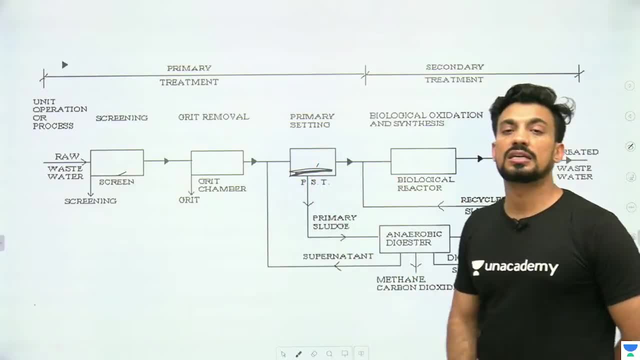 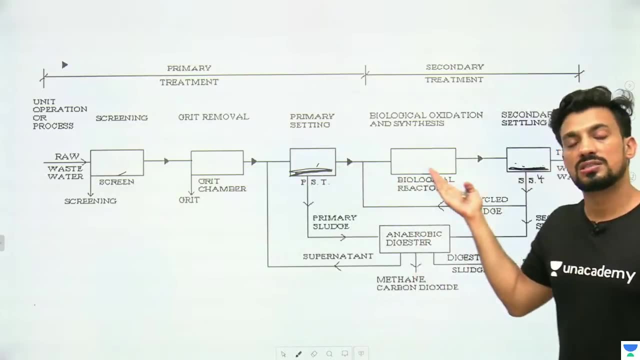 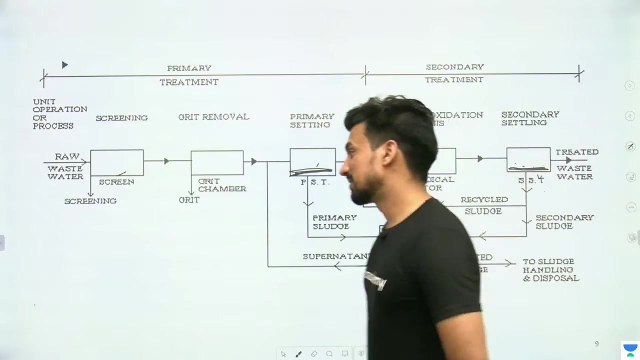 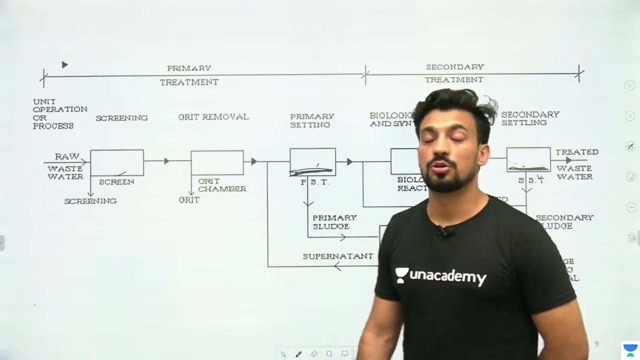 They took some sludge from here and put it here so that the amount of bacteria or biomass is increased here. more bacteria will be present, then it will work faster. it will decompose the waste faster. This is cheating. this does not happen, as it will settle in the green chamber. we will study the design of the great chamber. we will design the great chamber according to which we will do it. 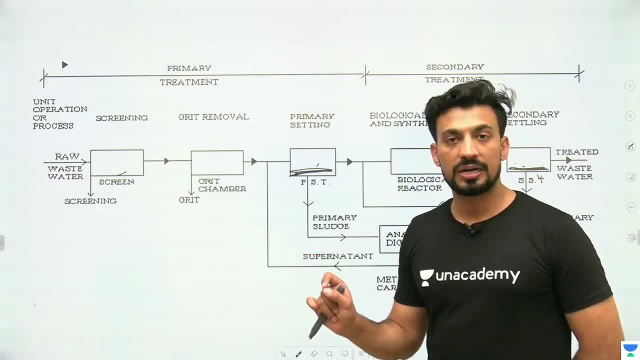 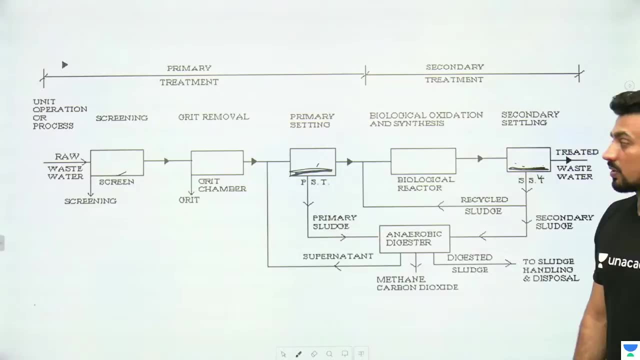 The nature of the particle is different, the specific gravity is different, So it's very difficult. The question is: how will it be solved? So we will design it in such a way that the organic does not settle here, So only inorganic will be there and organic will settle here. 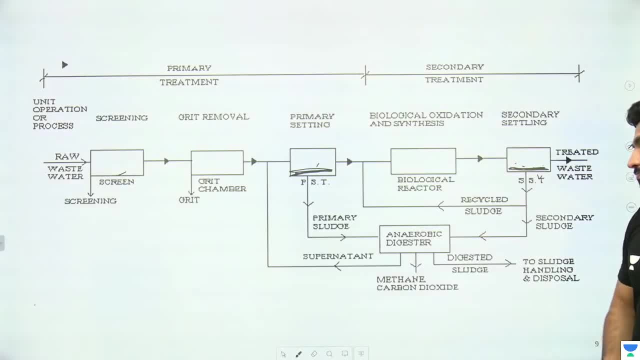 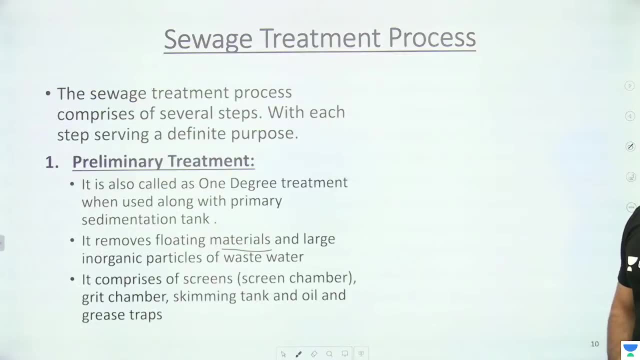 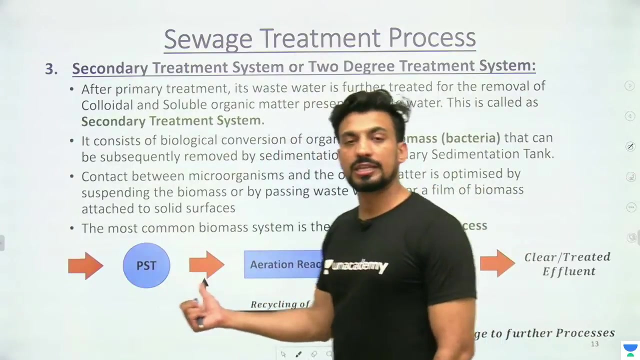 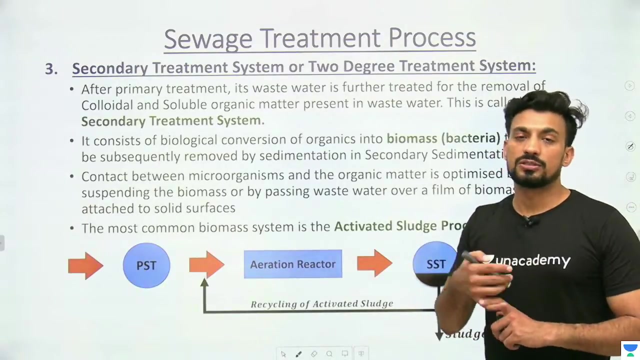 Let's move ahead. Next Now come to the secondary, After the primary sedimentation tank. now this process has started. Before primary sedimentation tank, the floating material was removed in the screening In the grid chamber. any rock, stone or inorganic waste was removed. 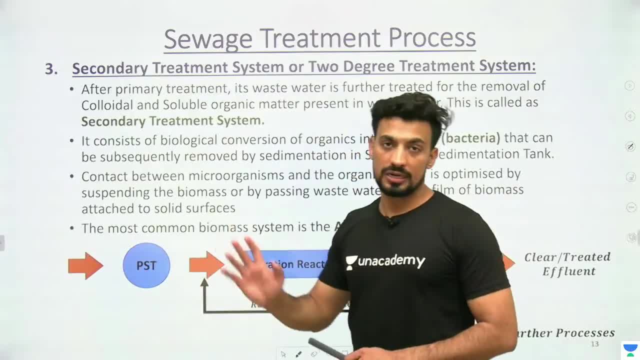 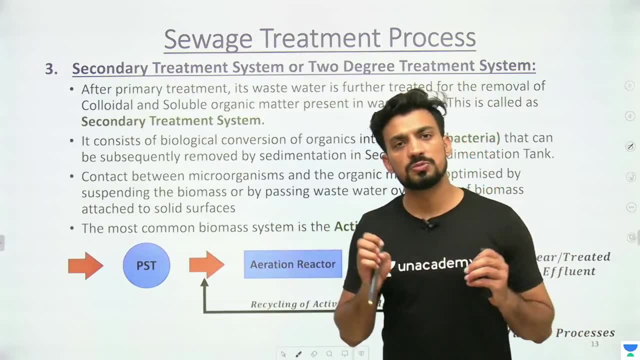 Now water came in the primary sedimentation tank, so 60 to 70% organic waste was removed here. Now you are sending that water in the aeration reactor. In aeration a lot of air will be present in it. A lot of bacteria will be present in it. 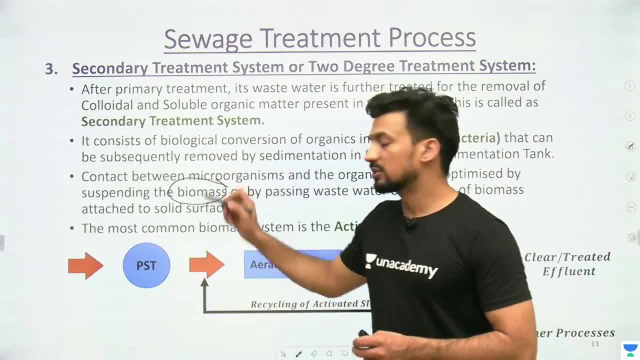 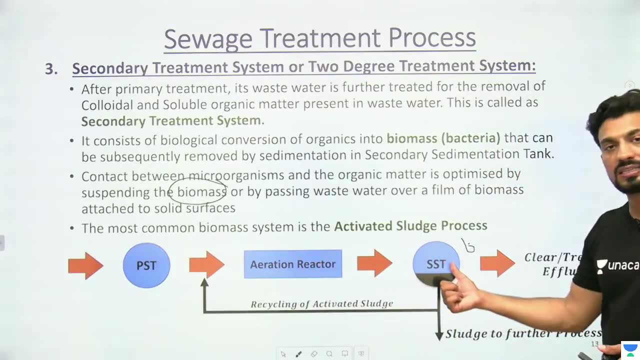 Which we call biomass. So what will be the presence of biomass and bacteria? What will it do? It will react with it and decompose the waste. After decomposing, this water will go to the secondary sedimentation tank. This sludge will sit down there in the tank. 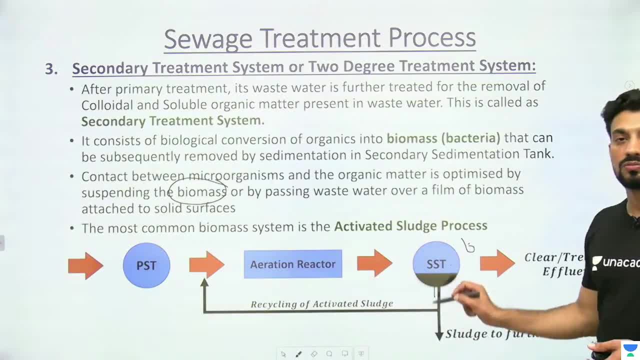 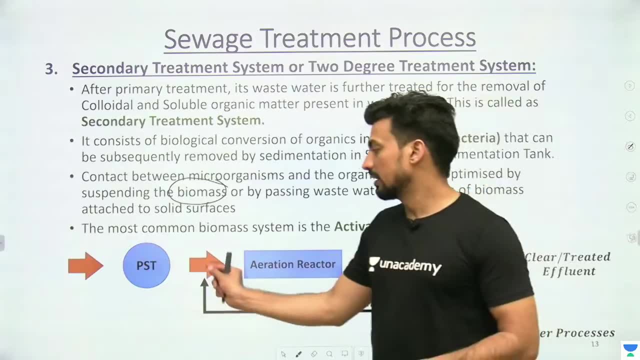 And what will happen after that? You take the sludge out of here. What do you have to do with the sludge? What work do you have to do? And bring some sludge back from here and add it here in this process? 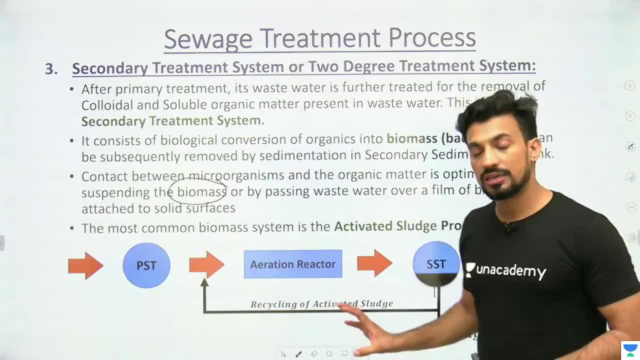 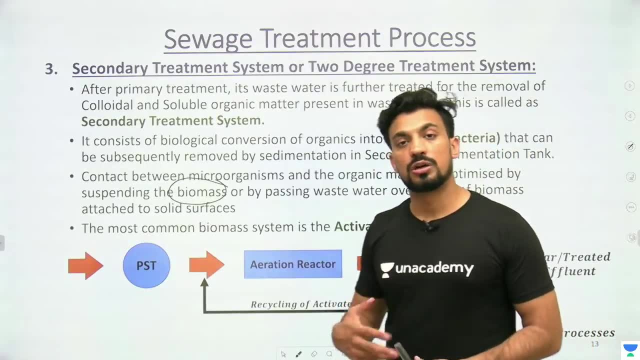 Or put it in the primary sedimentation tank So that a lot of bacteria comes in it, Biomass comes in it And as the water comes in it- As the water comes in it, By the way, its treatment will be fast. 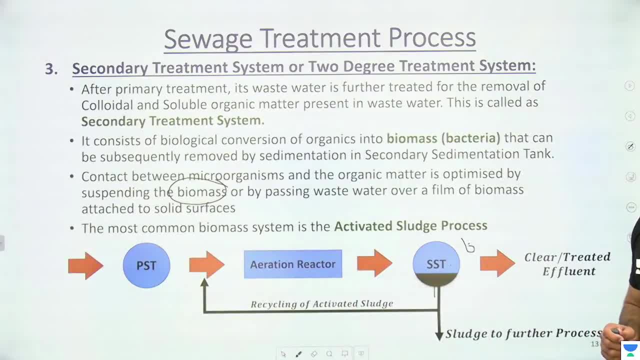 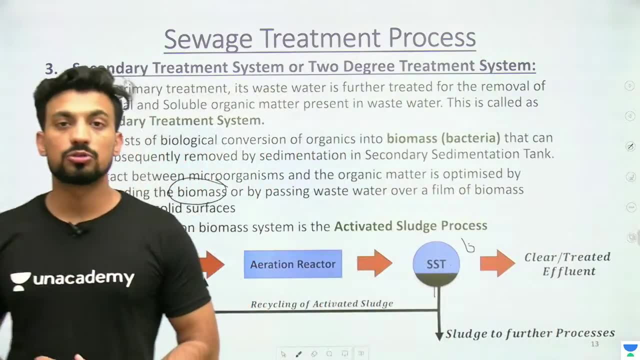 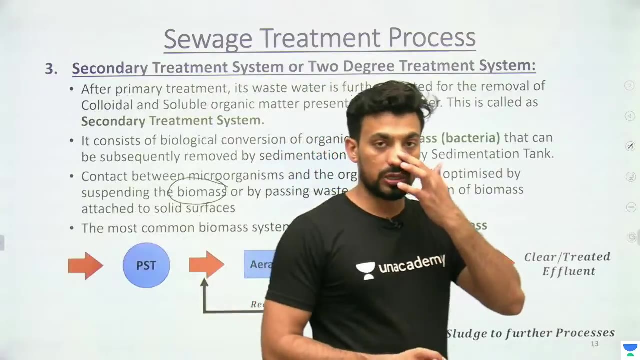 It will be fast here. First, organic particles are not done because organic particles are light. Their specific gravity is low. They will not settle quickly. Large size particles are inorganic. Remove the inorganic first. Inorganic particles will be heavy. 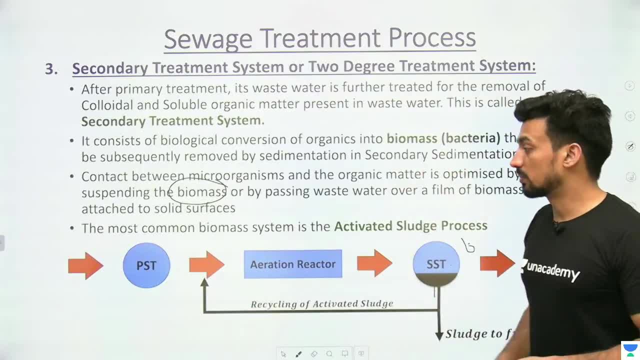 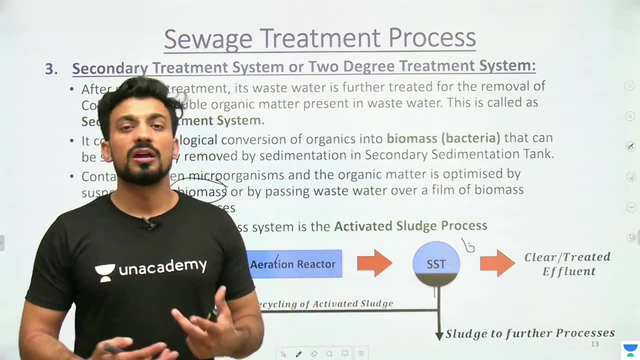 If you do not remove it first, You will say that we will take them with us. Then you will bring it here and here. These are your reactors. They will fail. There are so many heavy impurities, Why do you have to drag them forward unnecessarily? 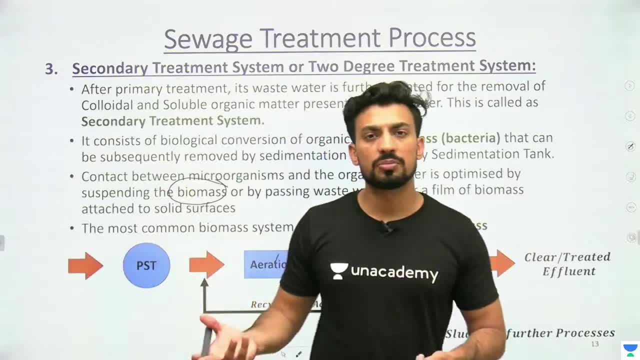 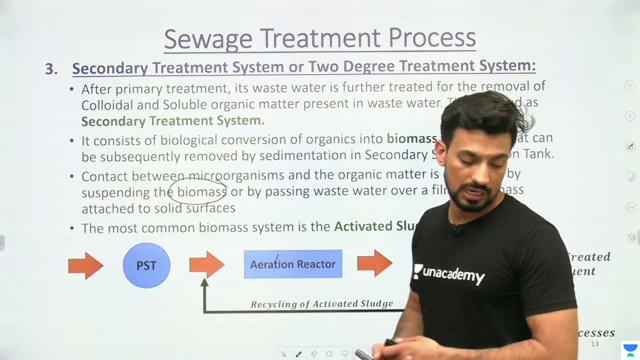 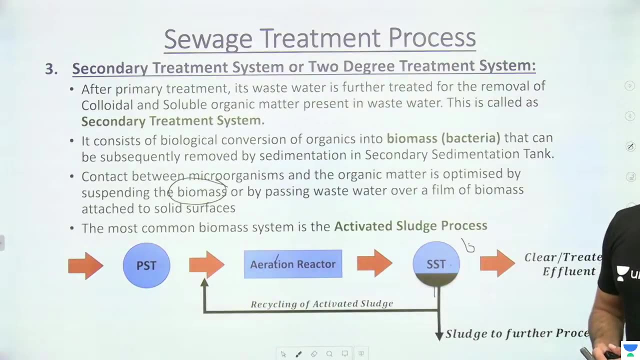 Separate them first And throw inorganic waste, rock and stone anywhere. They will not cause any harm to the environment. Any construction is happening, Use it anywhere. Use it in filling wherever. If you are sharing it with your friends, To remind them that you are a very good person. 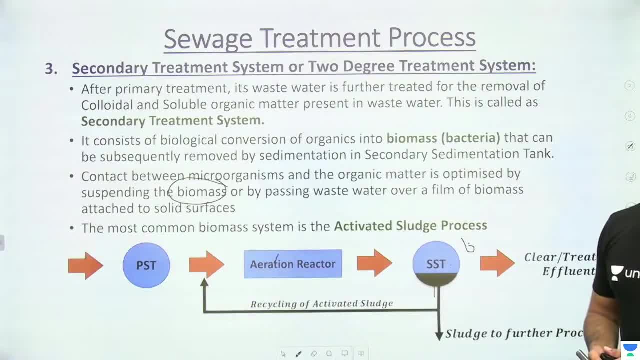 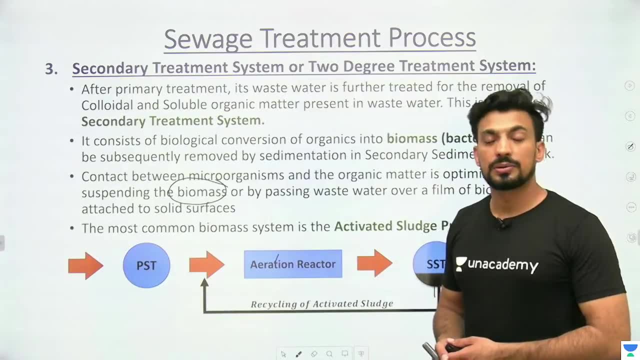 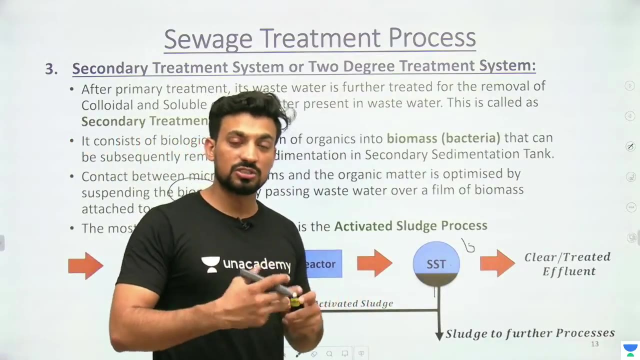 That's it: you are a very bad person. Sludge, Sludge, Sludge. A bad example is: You have friends. You tell your friend that he is a very bad person. Ok, One is waste: When the waste is concentrated. 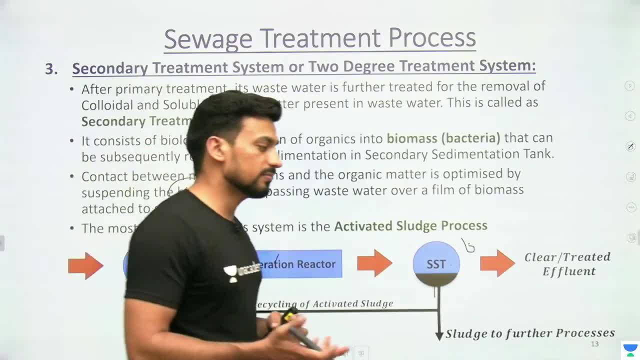 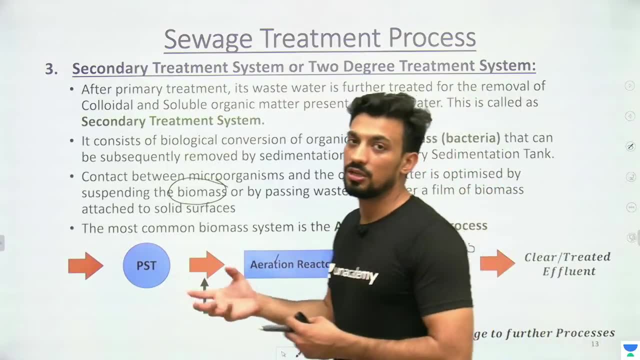 What you have done and as you talk, You are talking. You are talking about anything. This person is very good, this person is a very good person. he is a very good person. he is a cream man means it is completely good. concentrated here. 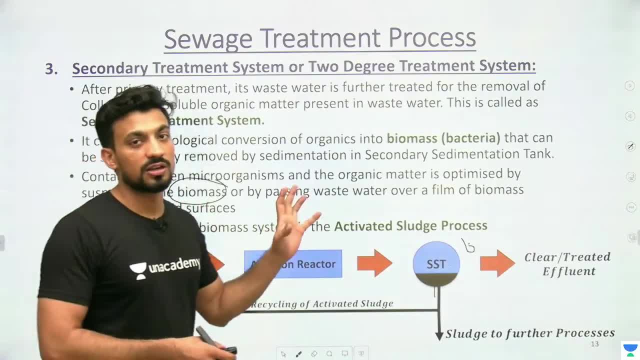 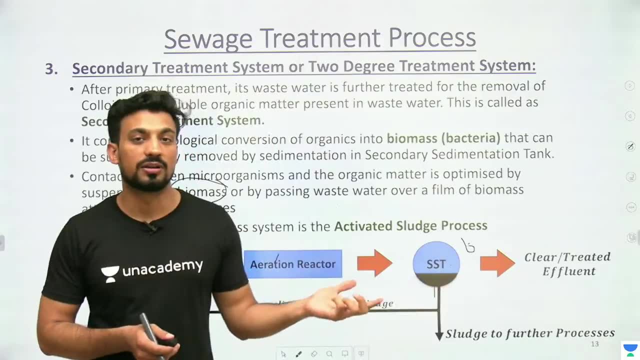 In the same way. what do you tell your friend? that there is one thing that is waste water. one thing is that when all the impurities of waste water are oxidized, you have completely concentrated them in the form of sludge. So what is that? That is not your dear friend. 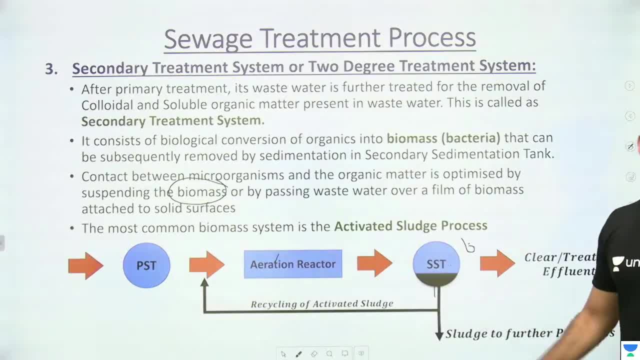 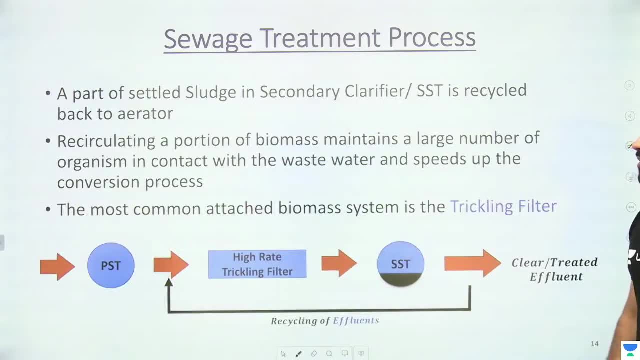 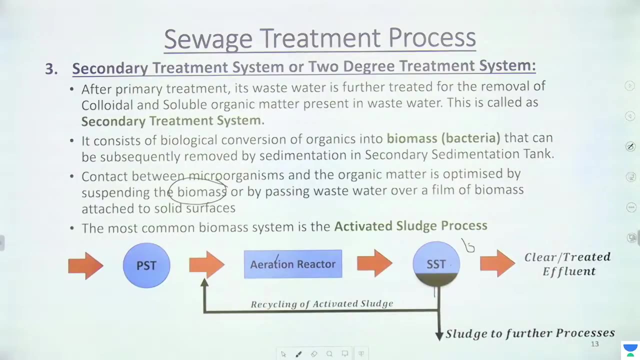 I am just giving an example. I am telling how you have separated the particles from the waste here. Come on, let's go ahead. Apart of settled sludge, this whole story is written in the same way in English: After the primary treatment, its waste water is further treated for the removal of colloidal and soluble organic matter. 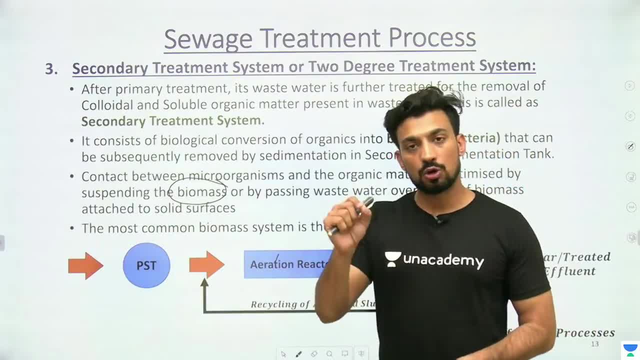 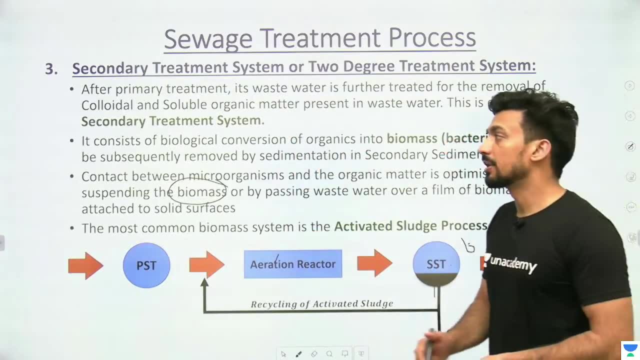 The particles that were not settled, which were soluble. mixed or colloidal means they were not settling in the water. So what will we do to them? We remove them in the secondary treatment. It consists of biological conversion of organics into biomass. 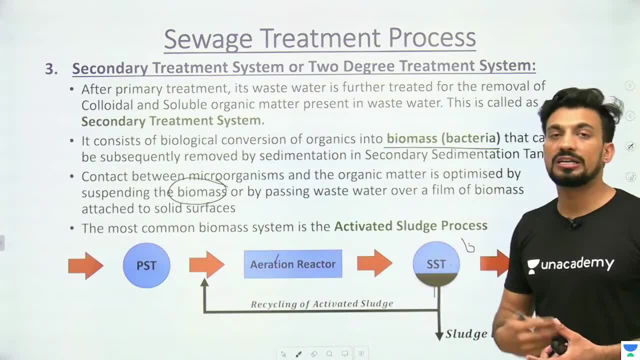 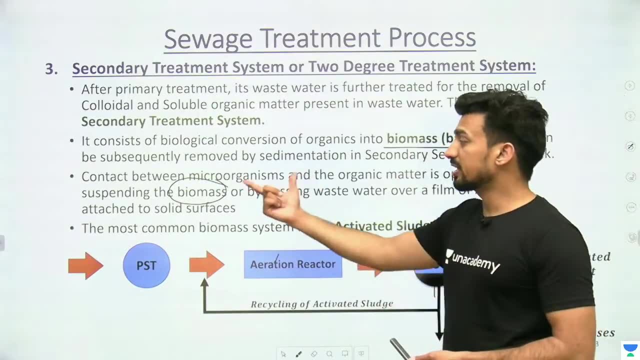 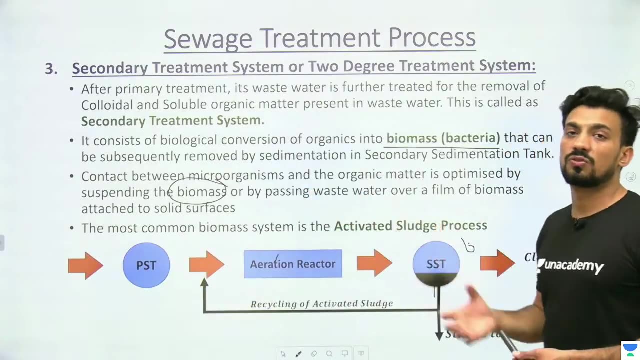 We convert it into biomass, We decompose the rest with bacteria And then they will come here and settle here, And the contact between the microorganism and the organic matter is optimized by the suspending biomass And or by passing waste water over a film of biomass. 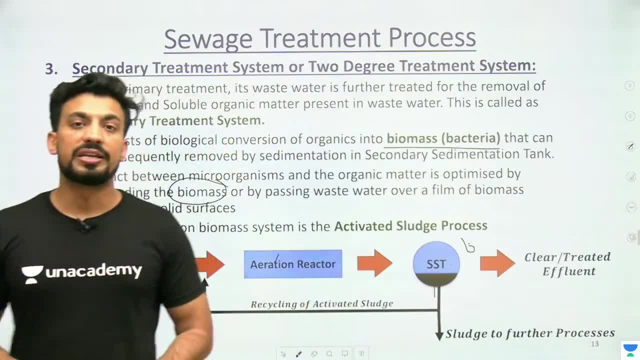 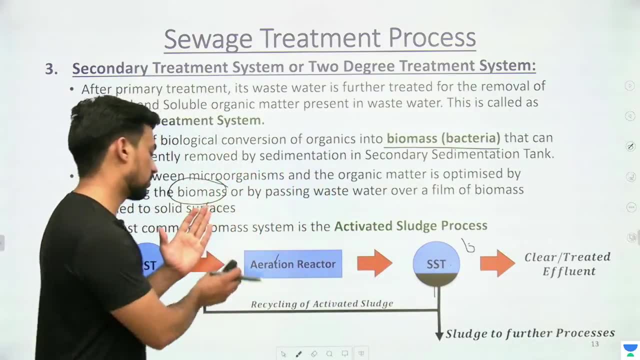 I have already told you that it has to be brought in contact with bacteria. Now, if you want to put bacteria here, put bacteria on a whole tank or on a surface, And this waste water here On that surface, So do it that way. 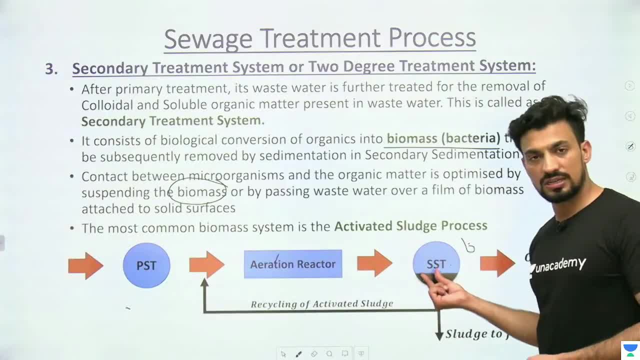 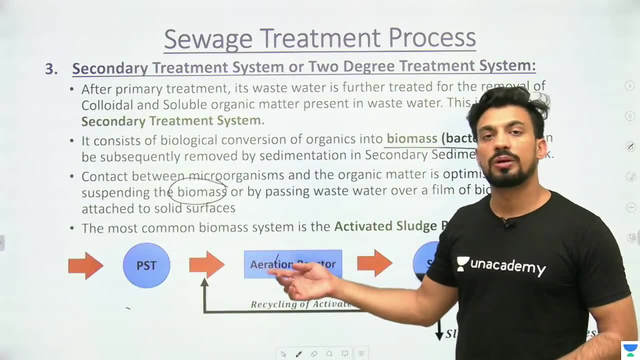 Ok, the one who sends behind is that: pick up some sludge. There are a lot of bacteria in this sludge. Pick it up and put it here. This means the bacteria is introduced Now that bacteria will continue to multiply here itself and decompose the waste quickly. 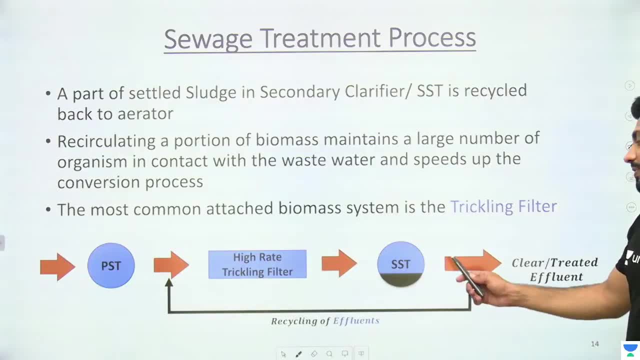 A part of settled sludge in secondary clarifier or secondary sedimentation tank is recycled back to aerator. Recirculating a portion of biomass maintains a large number of organisms in contact with the wastewater and speeds up the conversion process. The most common attached biomass system is known as trickling filter. 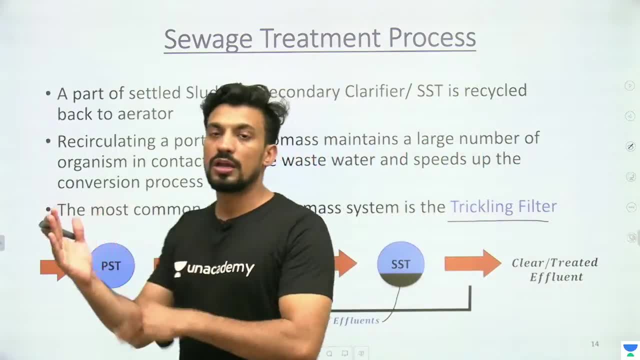 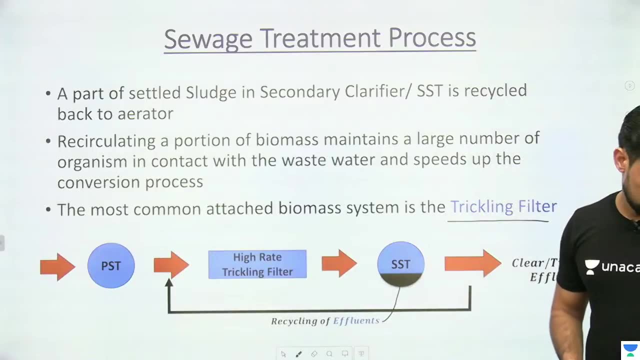 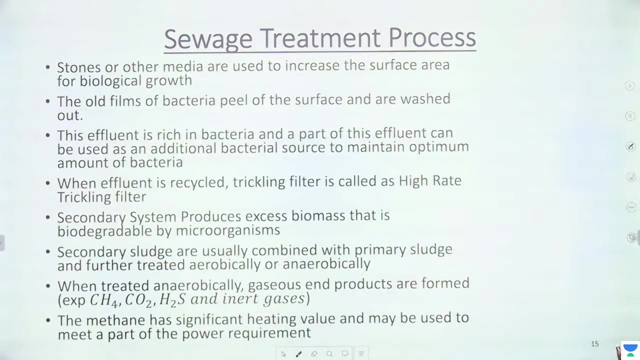 Attached means you are throwing it on some surface. You take it in contact with some surface and throw it. This is an attached system. Let's move ahead. In the sewage treatment process, stones and other media are used to increase the surface area for biological growth. 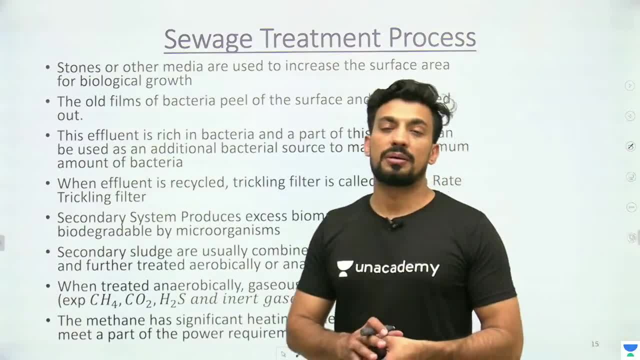 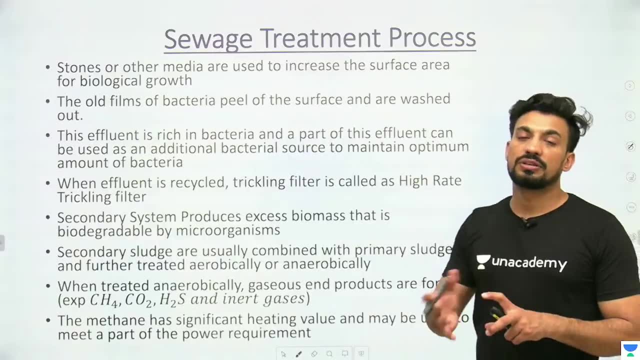 So whatever the sewage treatment plant is, or whatever filters are present there, stones will be present in it. Whatever reactors are present there, stones will be present there. Due to stones, more surface area will be exposed, So the sewage will be exposed to bacteria. 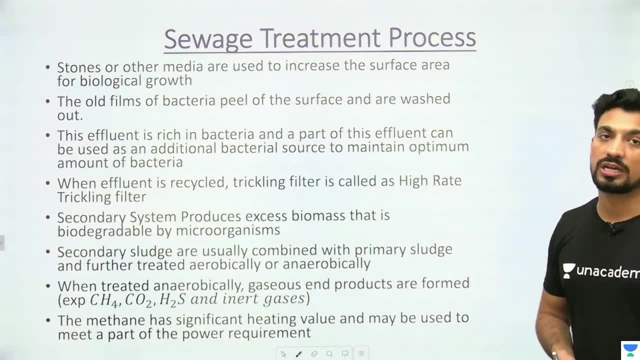 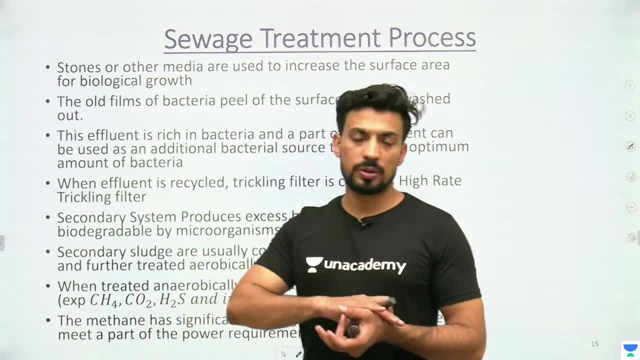 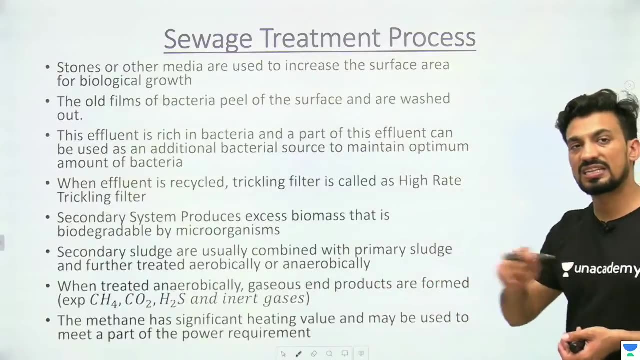 Due to this, the sewage will decompose it quickly. As it decomposes it, the layers that will form on it, the organic matter of the wastewater will be on it. The bacteria has decomposed it and its layers have formed, and later these old layers will peel off from it. 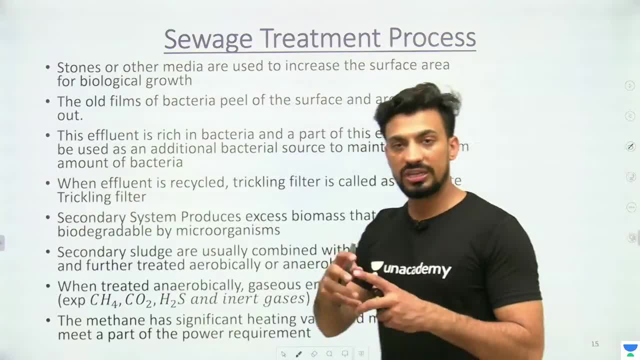 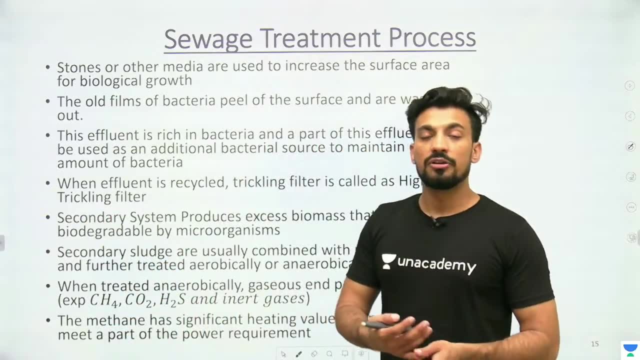 Affluent means liquid. When you are treating wastewater, the things which goes out are effluent. Those which are coming inside are effluent. The water coming in is the influent, Just like the input and output. the water coming in is the influent. 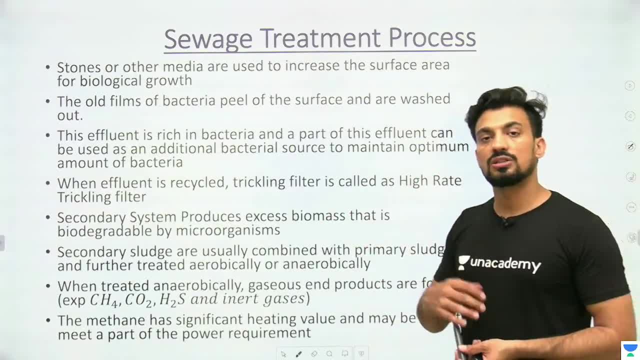 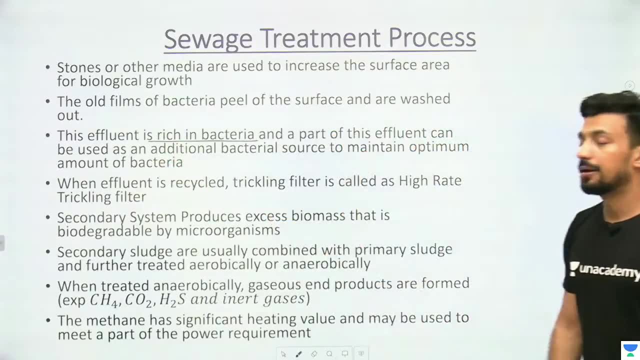 When it is going out, it is the effluent. That means if you separate the sludge from the waste, then you have that effluent. That effluent also contains a lot of bacteria. This effluent is rich in bacteria And a part of this effluent can be used as an additional bacterial source to maintain the amount of bacteria. 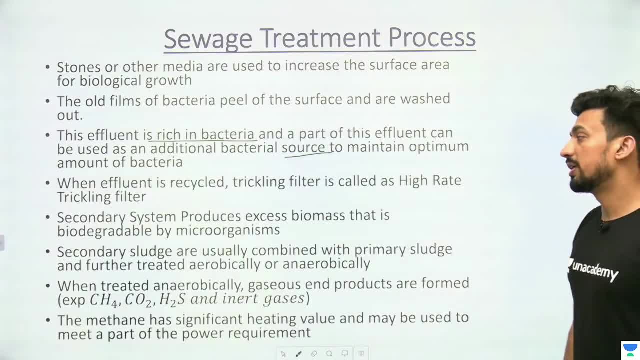 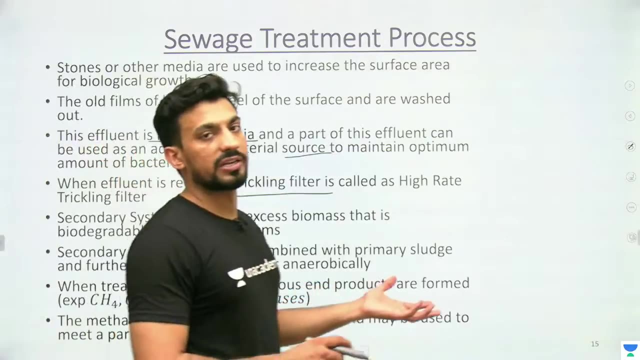 The same thing is happening here again and again After recycling the effluent. when the effluent is recycled, the trickling filter is known as high rate trickling filter. Filter means where you are reacting the microorganism with the waste. So if you add more microorganism, add more bacteria by putting the effluent in it, then you are increasing its rate. 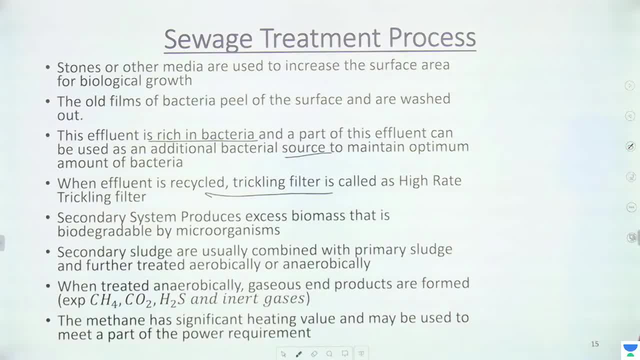 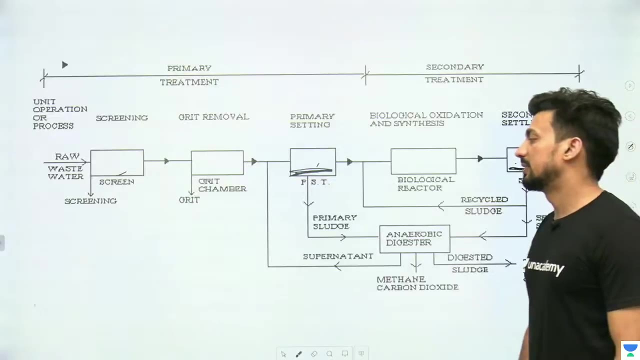 So high rate trickling filter is done. Secondary system produces excess biomass that is biodegradable by microorganism. Secondary sludge are usually combined with primary sludge and further treated Aerobically or anaerobically. Aerobic process or anaerobic process further. you can treat it. 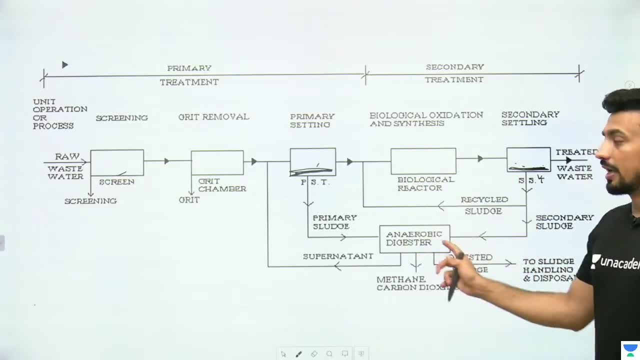 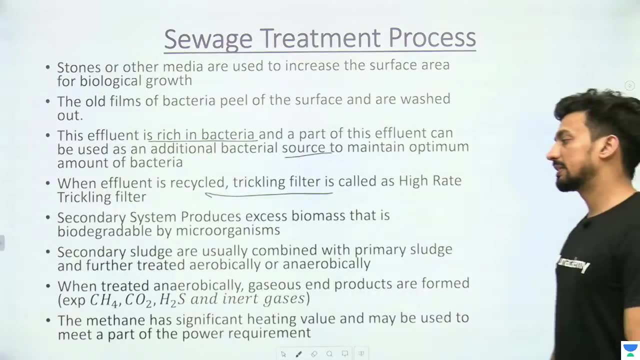 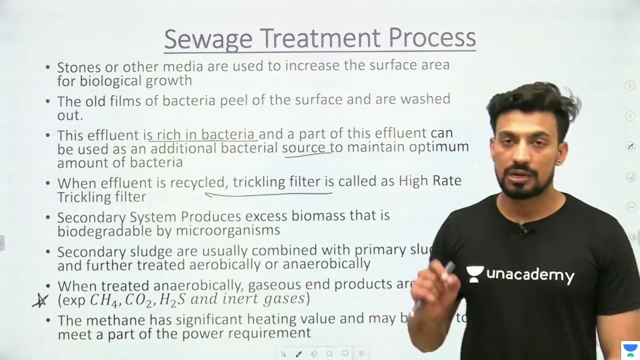 In the presence of aerobic air, you can treat it in the absence of anaerobic oxygen. When treated anaerobically, you will always remember that when we decompose the waste in the absence of oxygen, then gases like methane, carbon dioxide, hydrogen, sulfide and some other gases. 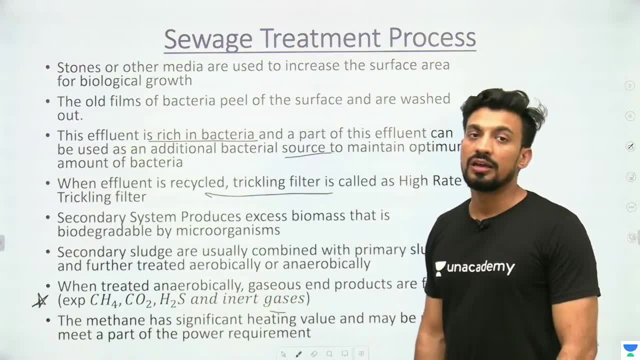 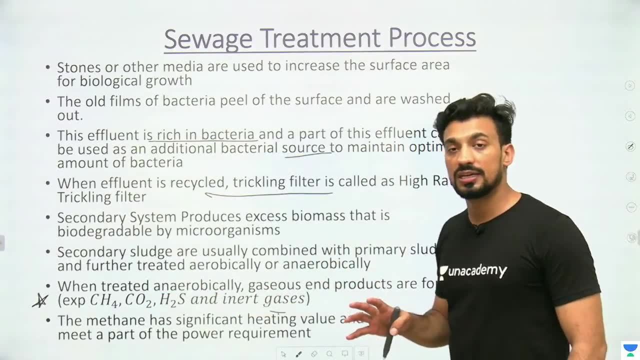 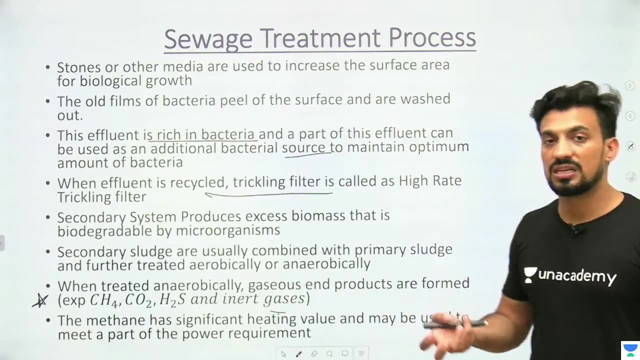 some inert gases. they are also released here. Now, whether you use them for energy, whether their bad smell pollutes our environment, then you will have to take care of it. So take care of it. and if you talk about methane, then we can take energy from it. 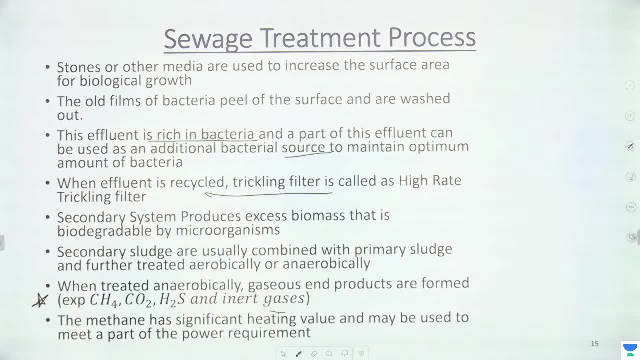 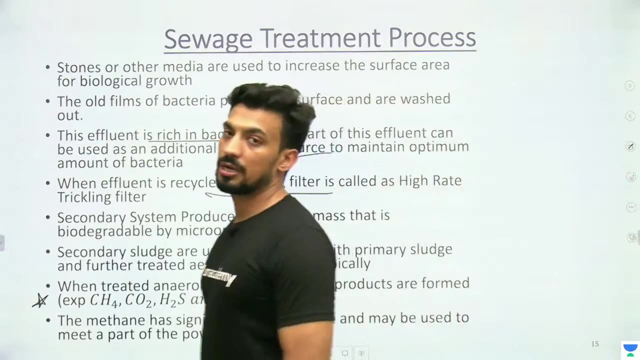 So we can use it too. Methane has high, significant heating value and may be used to meet a part of power requirement, So you can use methane. Which bacteria is there? We have already read about bacteria. What type of bacteria is there? 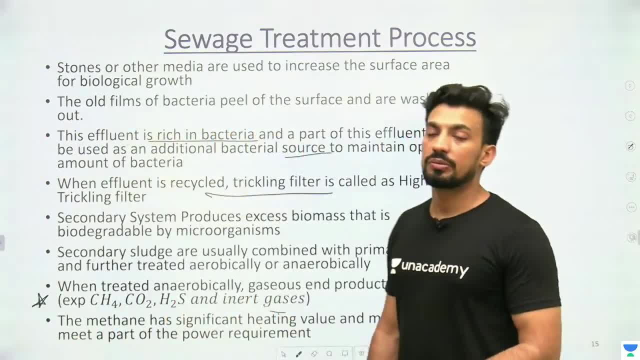 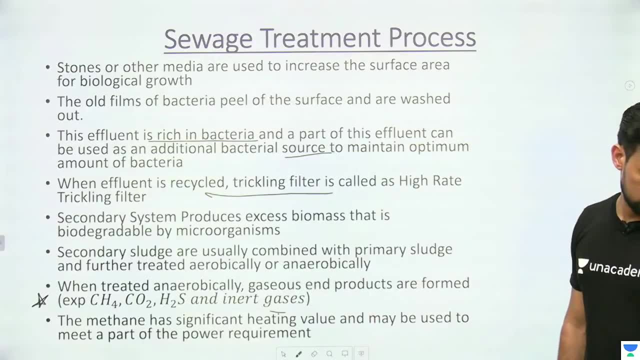 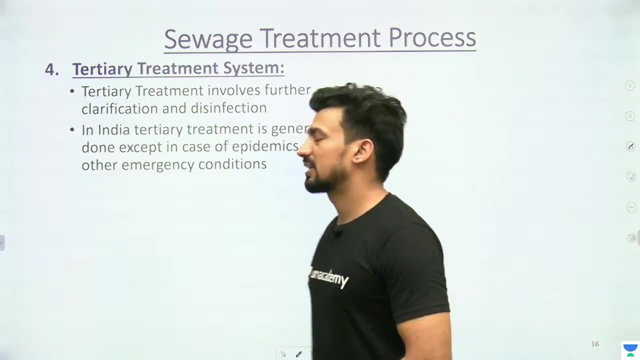 There are heterotrophs, autotrophs and facultative. We talked about facultative in the presence and absence of oxygen. We talked about phototrophs. So this is our talk. Then the tertiary treatment system. Tertiary treatment is not done much. 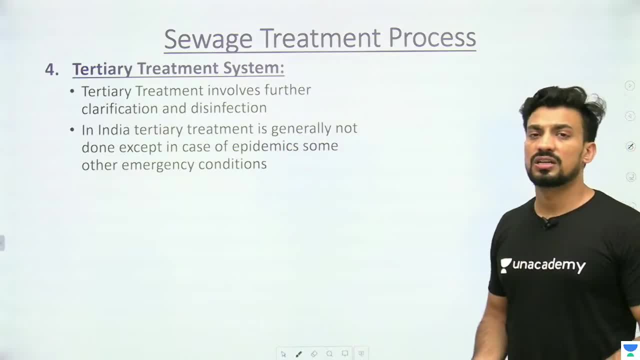 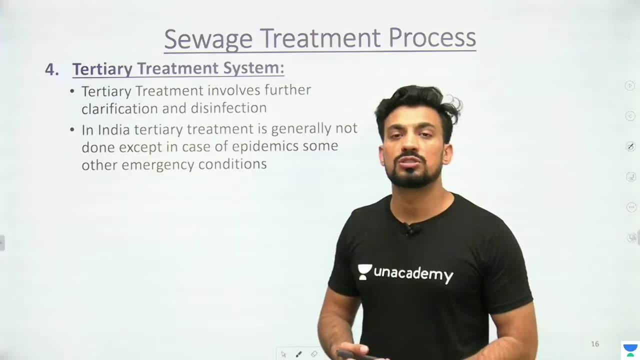 In the tertiary treatment process the wastewater is also disinfected. So this much is not necessary because there is no shortage of this much water So that the wastewater can be treated and used further for domestic supply. So disinfection etc is done rarely. 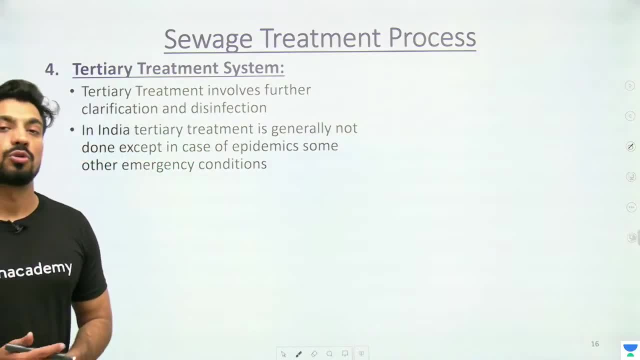 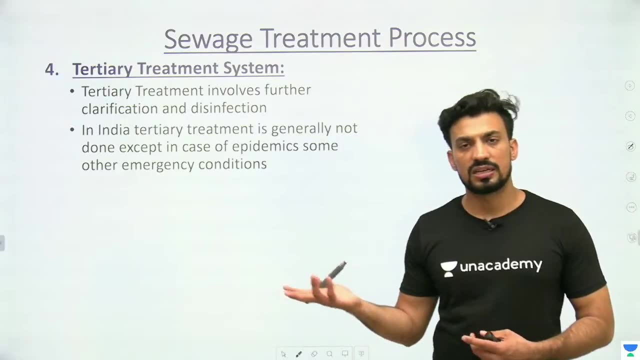 But in the case of epidemics, when an epidemic spreads or there is any other emergency situation, we can do it in that case, As it has not happened yet, God forbid tomorrow. Just take an example. Suppose such a bacteria started spreading through such a virus water. 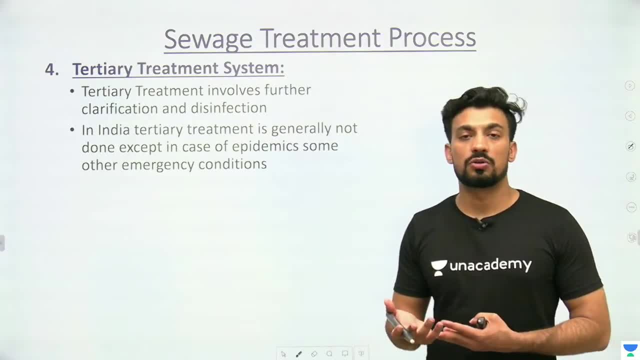 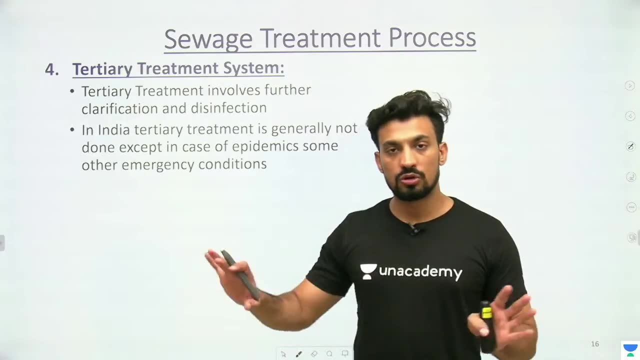 So it is also going in the wastewater. Why do we put a lockdown now? We put a lockdown so that those who are inside the house are safe, Those who have been infected outside the hospital or anything. they will be treated and the rest will be safe in their homes. 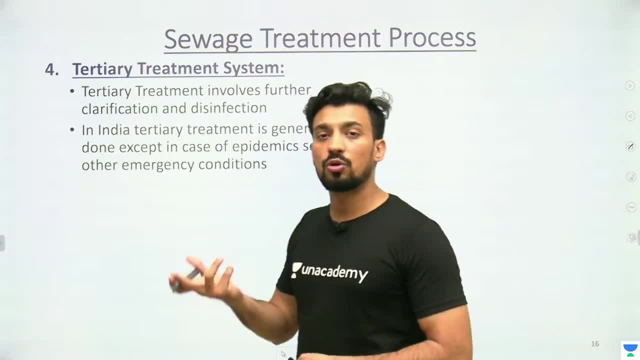 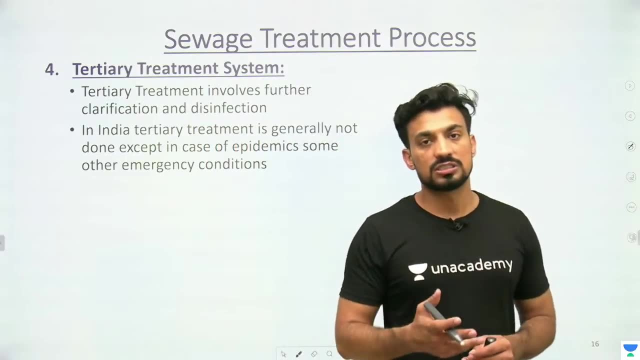 This is what lockdown means. In the same way, there will be a need to control that the wastewater, the clean water that is coming to the house. it is definitely taken care of that it is not a pathogen and it is disinfected. 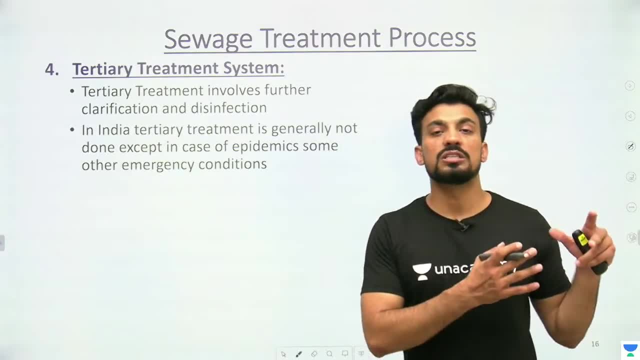 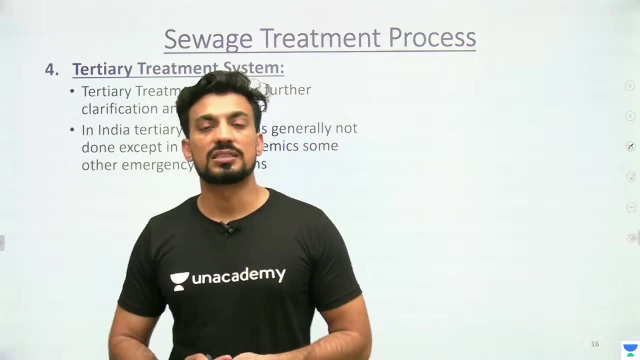 And then even if someone is going from somewhere, infected water, from any society or locality, it is also going to the infected wastewater, then it will also be treated If such a situation comes- epidemics or any such emergency situation- due to which the wastewater is also creating further problems. 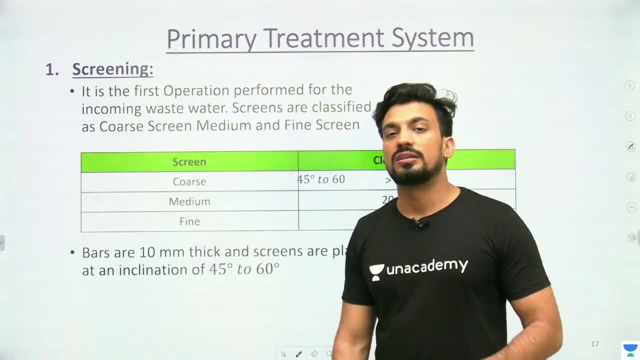 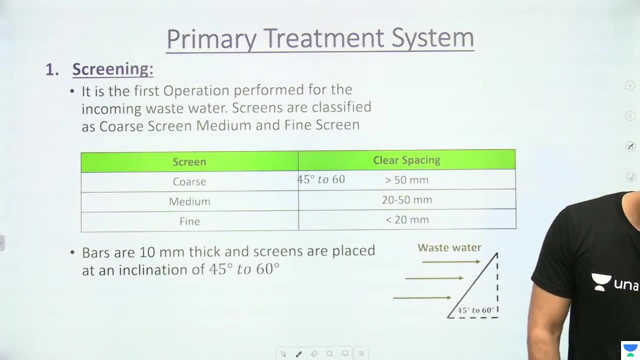 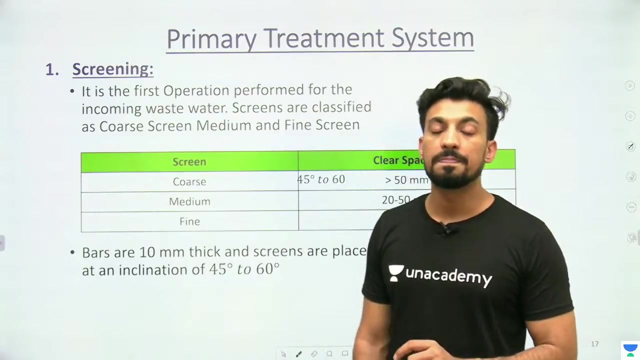 then they will be needed there. Otherwise, tertiary treatment is generally not done. Let's talk about screening. See, it is like this: No one is taking the name of the virus, But the truth is some people are still thinking that covid cases have gone down. If covid happens once, then its effect does not last for long. Your body will recover once. Covid test will also come negative, But it will take so much time to recover the body. There will be such side effects, there will be such issues that you yourself do not understand. 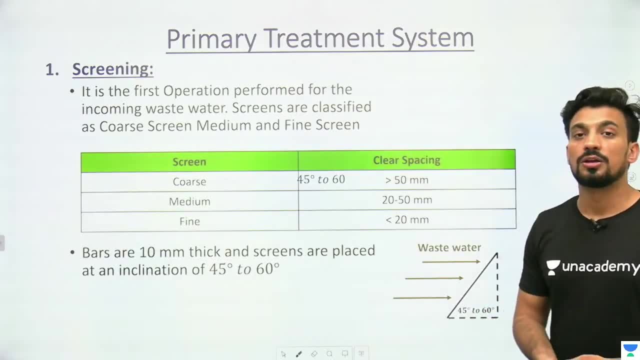 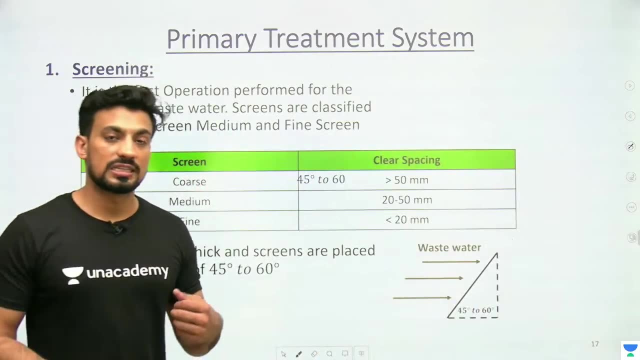 And how much has been spread in the world, how much research has been done on it. So you get to see some different effects everywhere. That's why keep things in mind. The third wave, which is, as expected, we were talking about September. 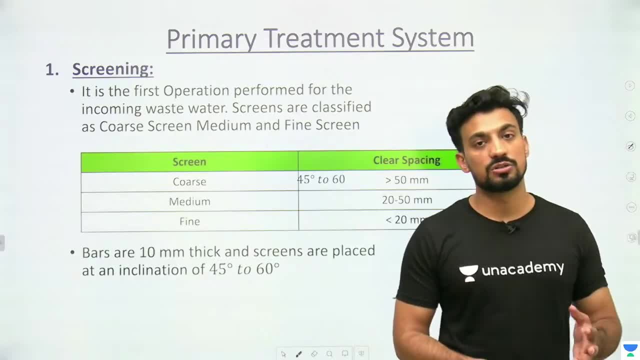 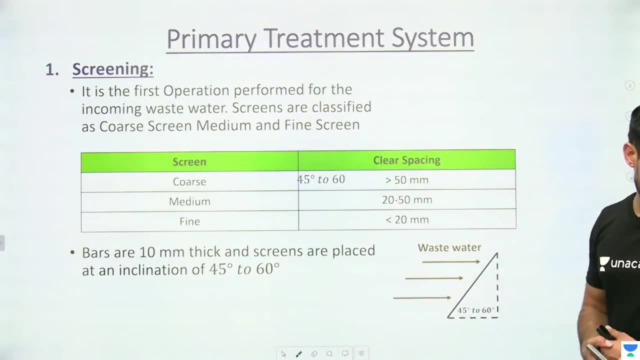 is also coming earlier than that. A lot of delta variant patients have been found, So that's why keep things in mind. We should not take things so lightly. Let's talk about screening. So what are the screens you have, According to coarse, medium or fine size? 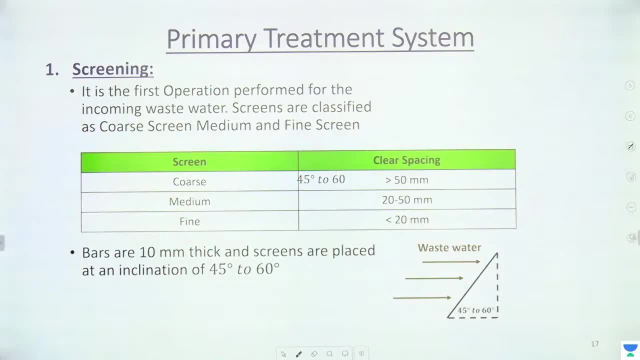 they are of different sizes. If the spacing between them is greater than 50 mm, then you call it a coarse screen, If it is between 20 and 50,, then medium, And if it is between 20 and less, then you call it a fine screen. 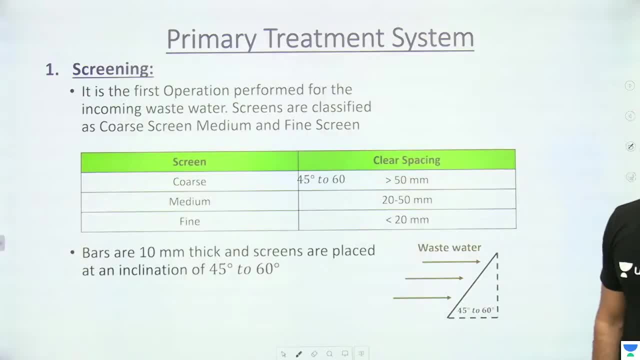 Then what will you call it? You call it a fine screen. Bars are 10 mm thick and screens are placed at an inclination of 45 to 60 degrees. 45 to 60 degrees- we provide them at an inclined angle And the size of the screen. 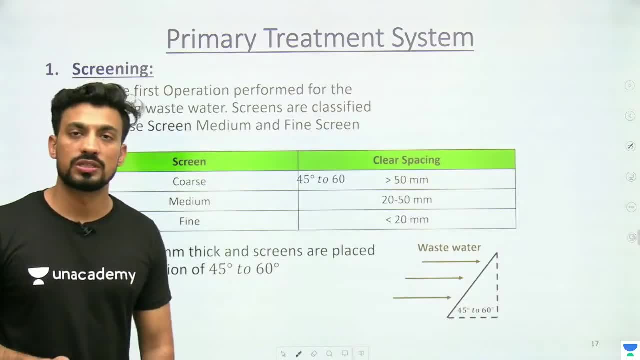 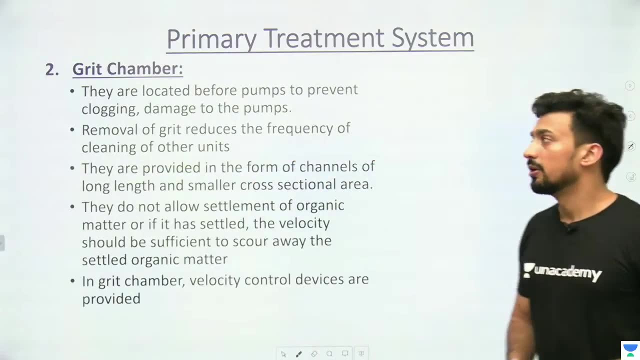 the smaller it is, the sooner it will be clogged or blocked. So we use big size screens so that the big waste can be removed from there. The rest will be removed further in the grid chamber. So if we talk about the grid chamber, 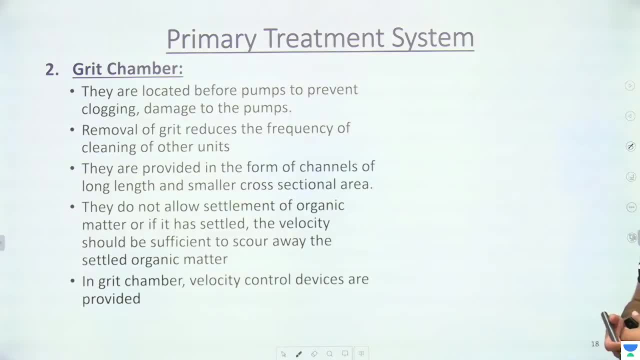 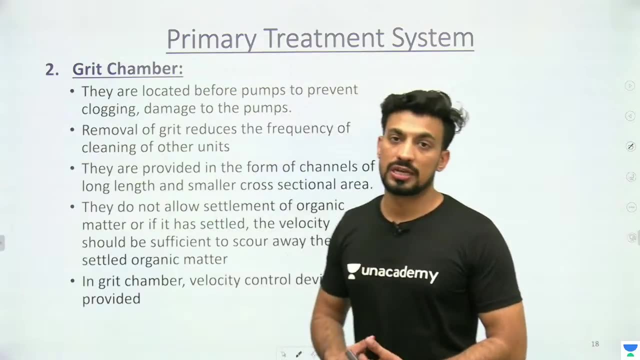 then what is the grid chamber? Grid chambers are located before pumps. They will be before the pump because if the concrete, stone and inorganic waste goes into the pump, they will spoil them, they will cause damage. So you use them before the pump. 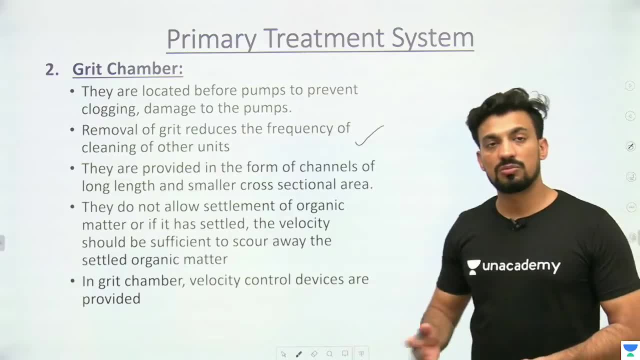 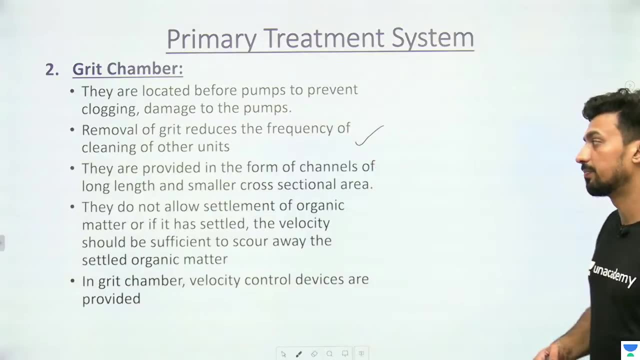 remove them so that if this waste is removed, then the maintenance of the units in the future will be easy. The heavy waste will not go into them, which we are removing from here. They are provided in the form of channels of long length. 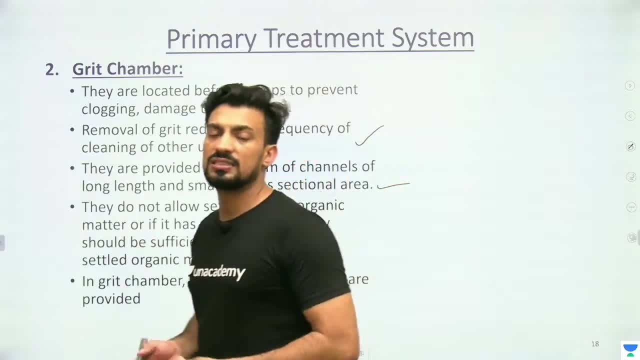 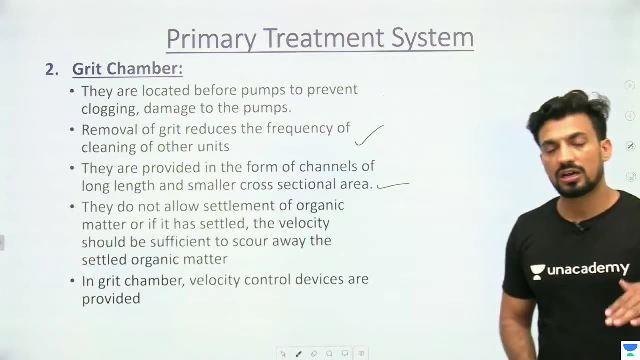 and smaller cross-section area. So you can say like this: the cross-section area will be reduced. we are making the water flow in the channels. The water is going into the small channels, so the concrete stone- whatever inorganic waste- is being settled there. 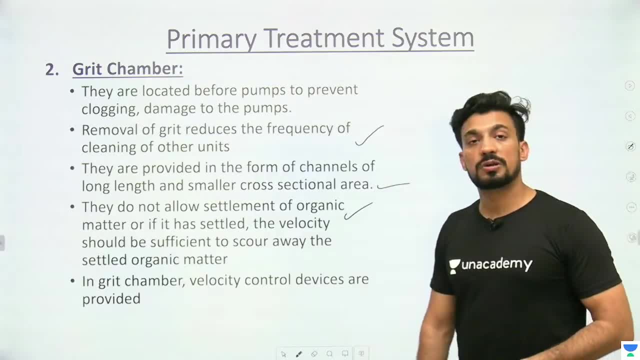 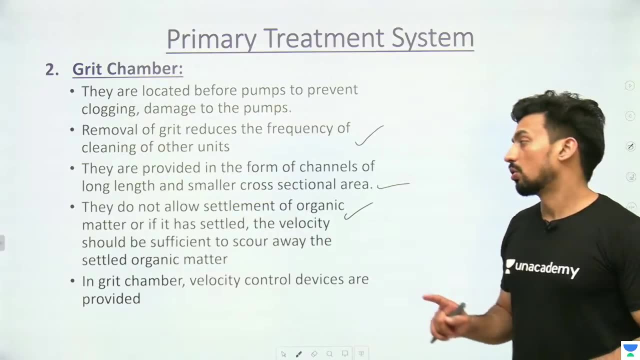 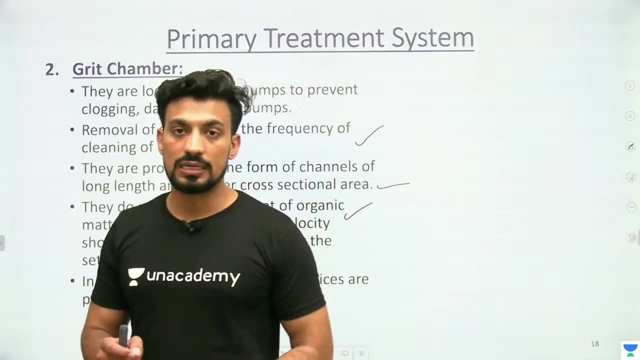 So the flow in these channels will be in such a way that only the inorganic particles are settled. the organic is not settled there. So the organic should not be settled. Even if it is being settled, then the organic particles are light. the specific gravity is less. 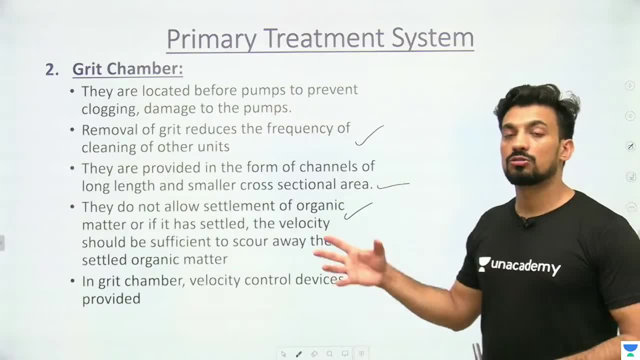 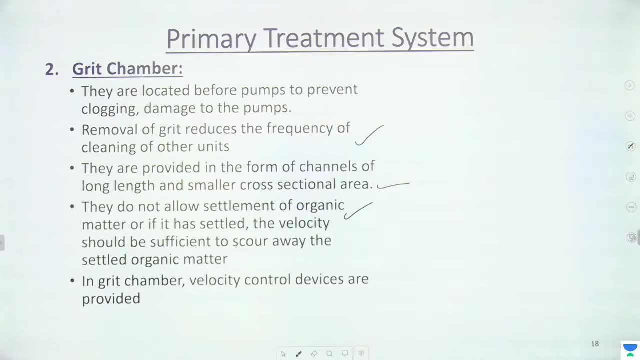 So increase the velocity of the water. So what will happen with that? Even if it is settled, it will be removed from there. the organic one will be removed. So in grid chamber velocity control devices are provided so that the organic is not settled. 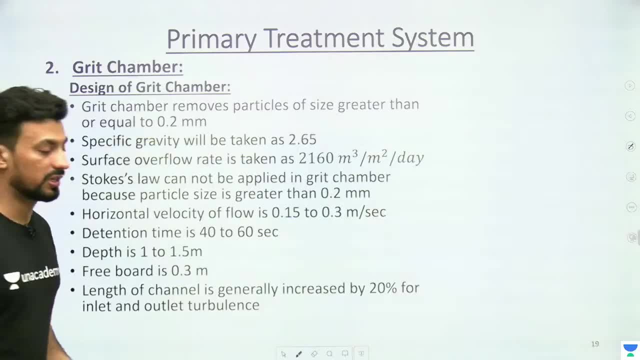 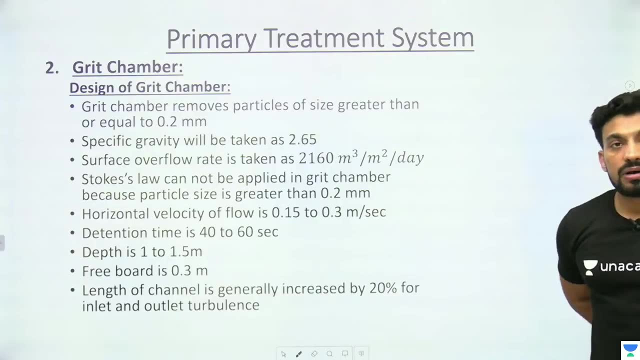 only the inorganic is settled here in the grid chamber, And let's talk about the design of the grid chamber. If we talk about the design of the grid chamber, then the first thing is that it removes particles of size greater than or equal to 0.2 mm. 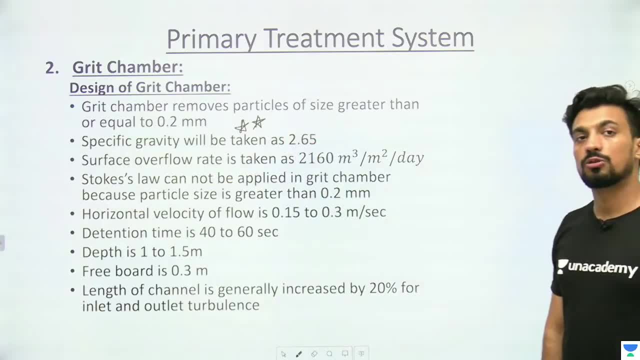 The first important thing is that the grid chamber removes particles of size equal to 0.2 mm or larger than that. Second thing: you consider the specific gravity, which is 2.65.. How much specific gravity will you consider? 2.65 of particles is important from the objective point of view. 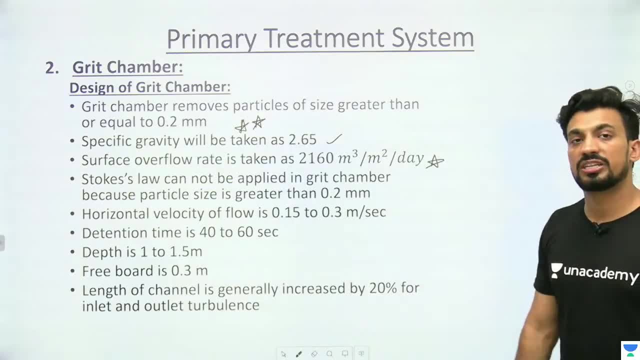 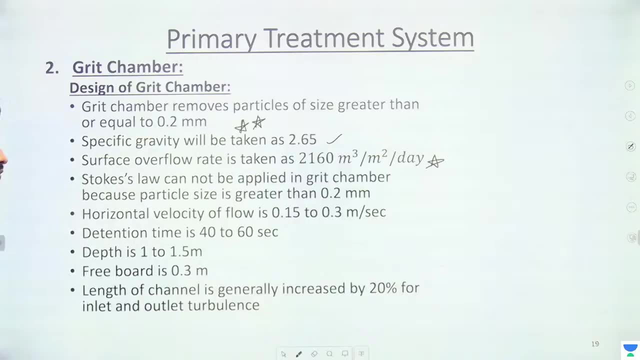 The surface overflow rate which we have already studied. in the sedimentation tank we consider 2160, 2160 m3 per m2 per day. You do not apply stoke slow. We talk about the size of the particle from 0.2 to 0.0002 mm. 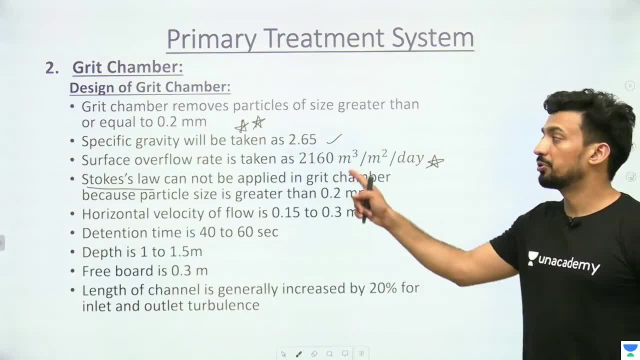 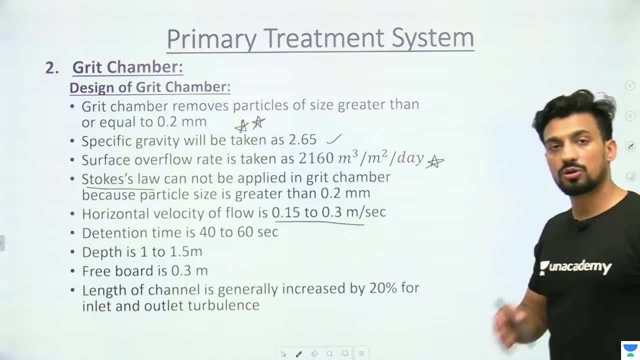 stoke slow. And here we talk about the size of the particle from 0.2 to 0.0002 mm. We are using the grid chamber for particles of size greater than 0.2 mm. The velocity of horizontal flow, or the flow of water, is 0.50 to 0.30 m per second. 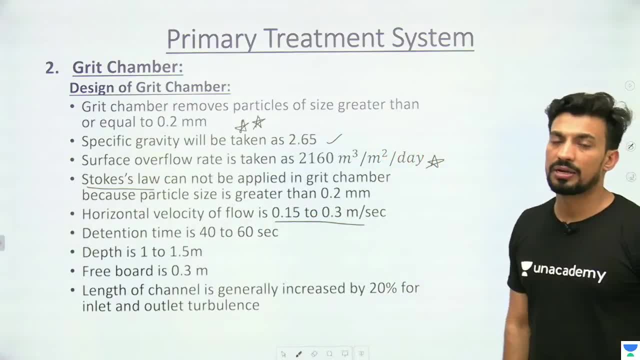 And the detention time. how long do we believe that the particle will settle there? Because it is an inorganic particle, it is heavy. it will settle quickly. We consider 40 to 60 seconds here. Its depth will be 1 to 1.5 m.